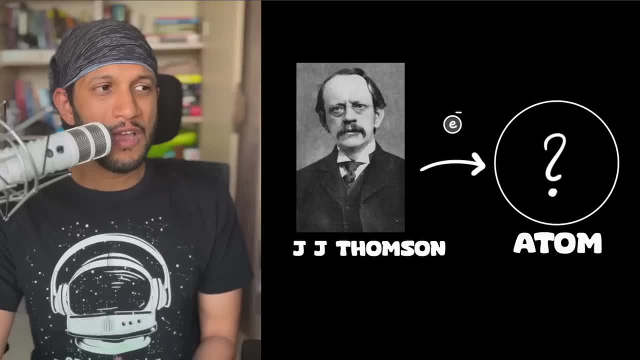 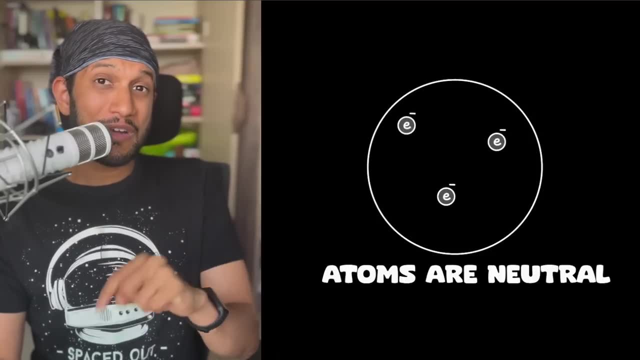 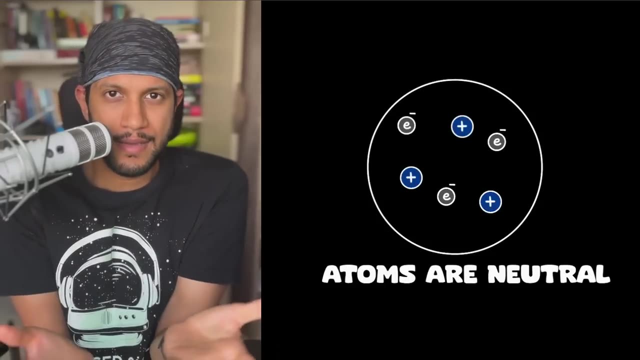 That is, figuring out what's inside the atom. You see, we already knew that atoms are neutral, right, But now we discovered that it has electrons, which are negatively charged particles, inside of it. This also means there must be some kind of a positively charged thing inside. 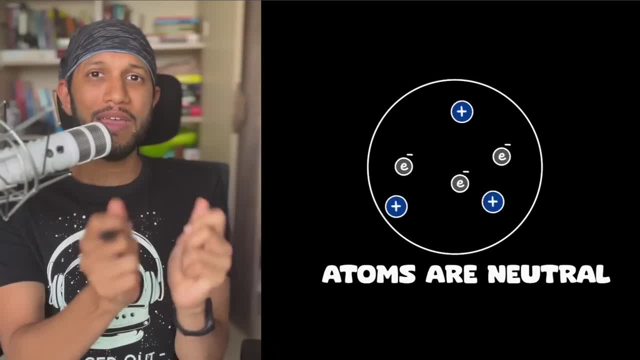 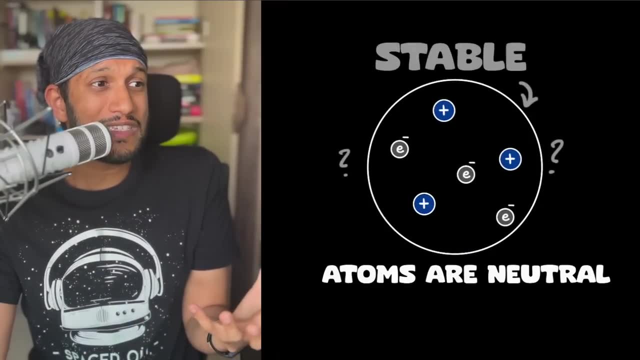 it as well. And they must be arranged in such a way that all their forces must get together, All their forces must cancel out, because they all attract and repel, And they must be arranged in such a way that it should remain stable. And so the big question was: what does that? 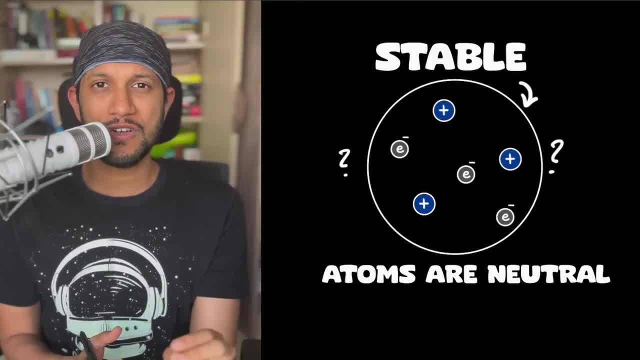 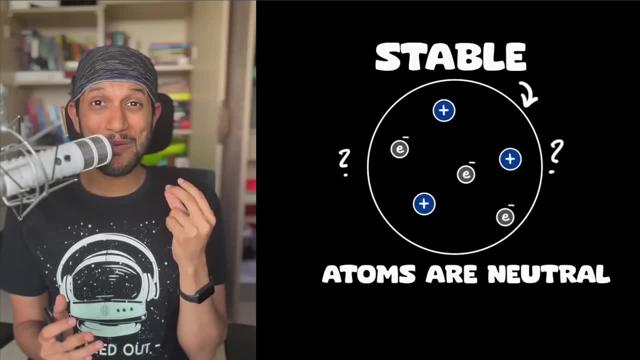 arrangement look like? What does the atomic structure look like? After the discovery of electrons, a lot of people were taking a crack at it And after a few years, Thompson came up with an idea and gave us the very first atomic model. How? Let's go back in time. 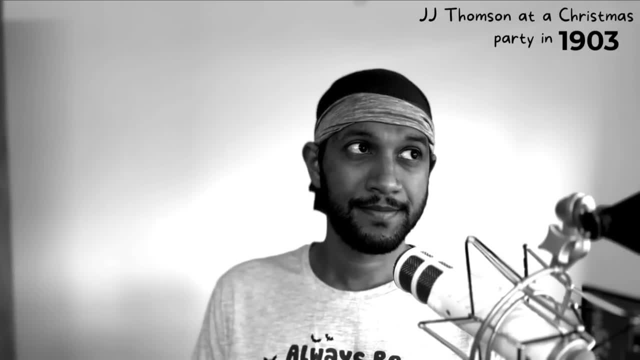 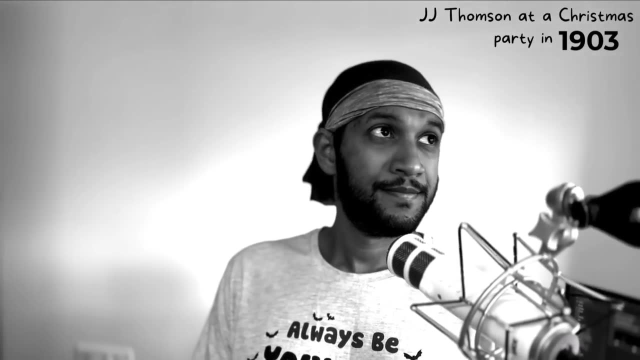 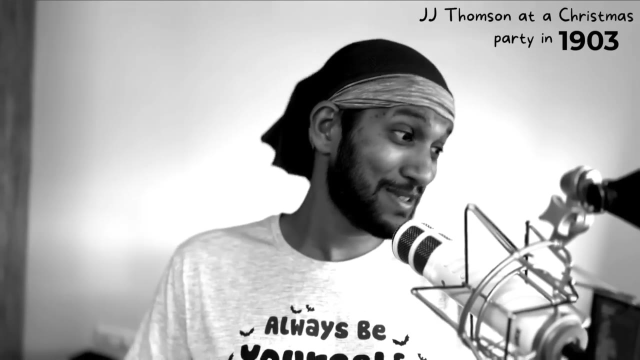 Oh my god, what a boring Christmas party. And what did I say? yes to this? Should I just stay at home and work on my atomic model? Oh my god, Enjoying the party, Mr Thompson, Oh, yes, yes, yes. Very nice, wonderful party. That's exactly what I was thinking about. 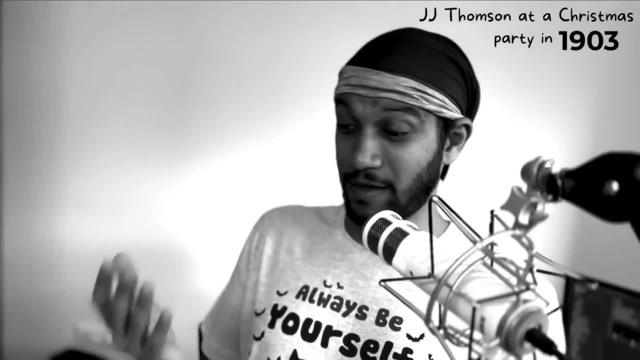 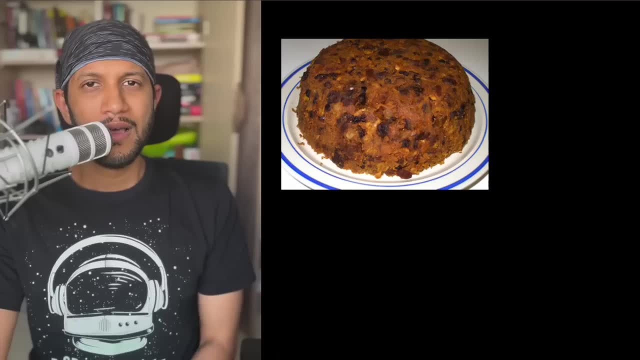 yeah, And how do you like the pudding? Oh the pudding, oh, that's incredible, yes, And then even the plums inside that pudding, oh, that is Now I'm not sure if that's really true. It would be so cool if it was, But what did Thompson? 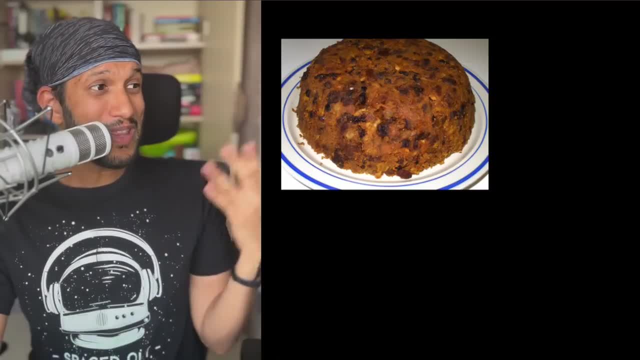 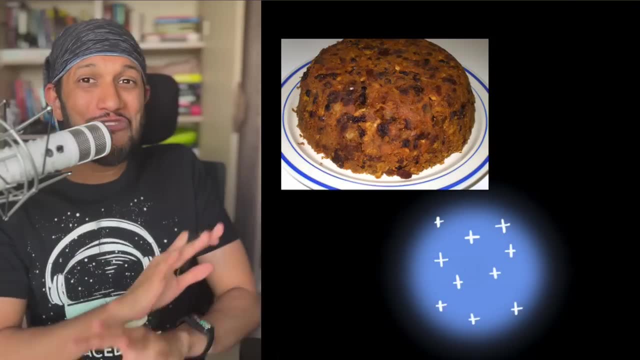 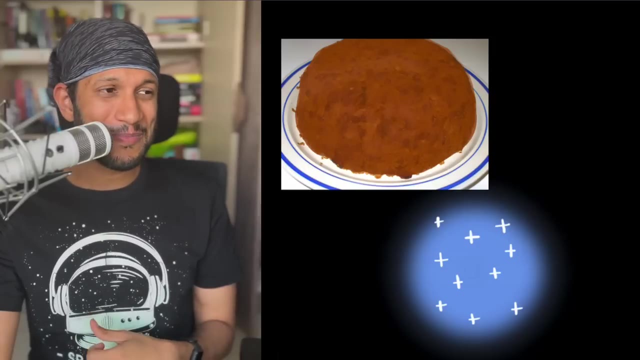 find out what was the idea that he got. well, he looked at the pudding and just like the pudding, he said that maybe the atom is made of a, some kind of a gas of positive charge that completely fills the atom up, just like this, just like the pudding part of that cake. and if we just had this? 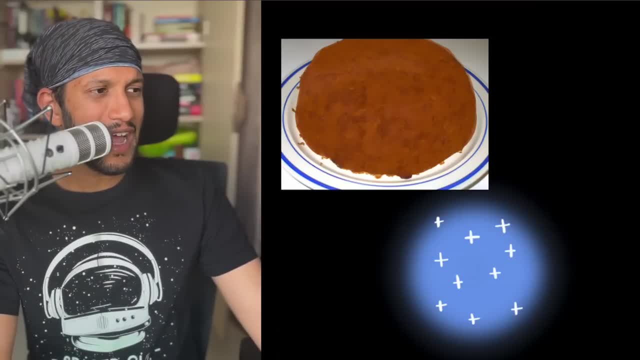 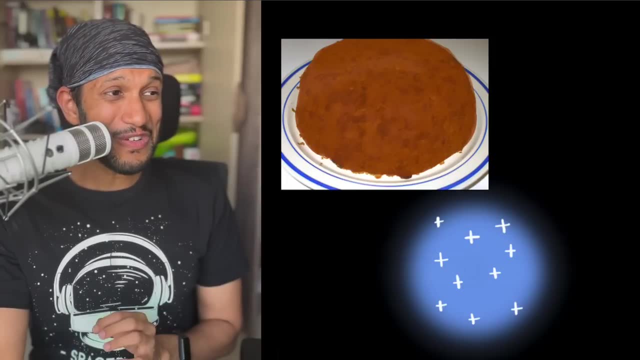 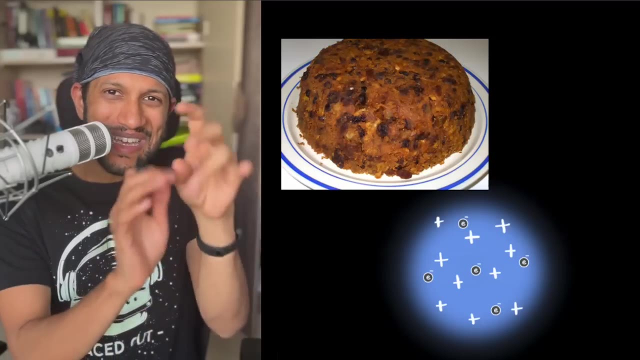 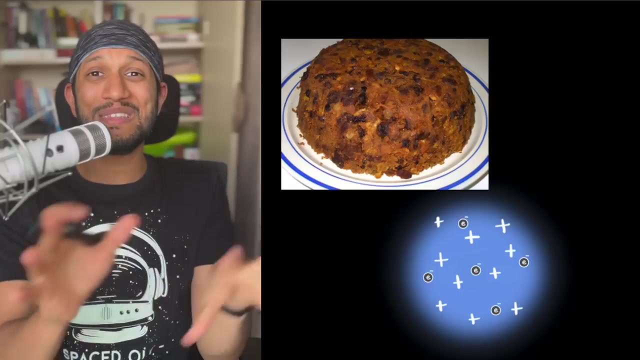 gas of positive charge, because positive and positive would repel. then that gas would tend to expand because positive, positive repels from each other. but what keeps it from expanding? the electrons. just like the plums in the pudding, the electrons are placed inside the pudding of the positive charge and the forces of the electrons and the positive charge all balance in such a way. 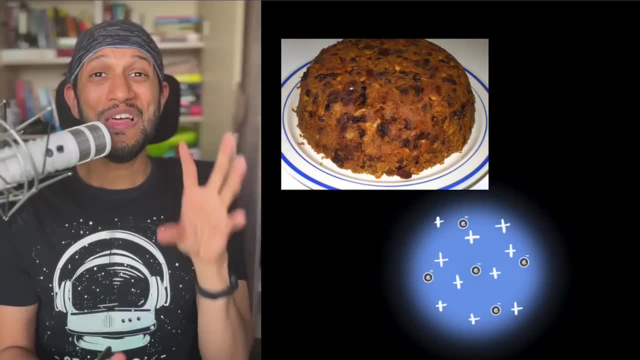 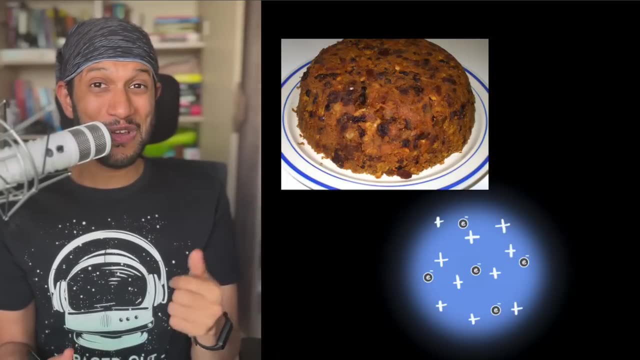 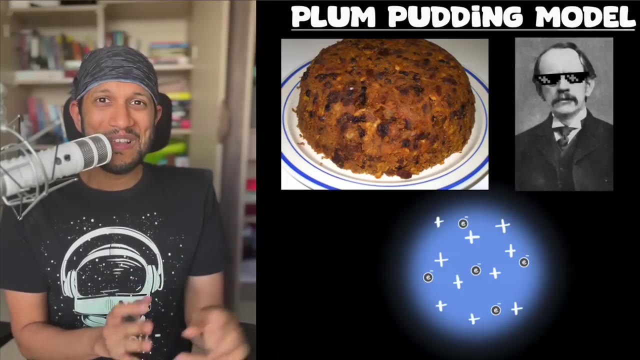 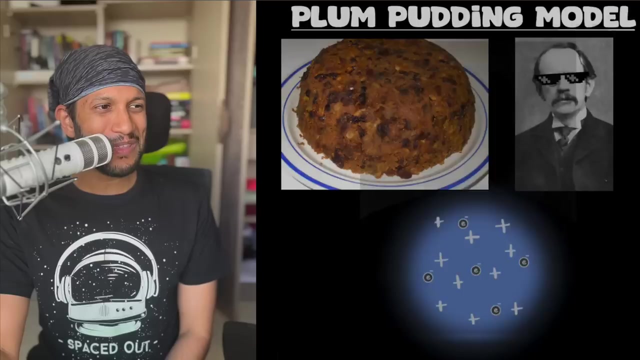 the atom stays stable. this was the plum pudding model given by jj thompson. thompson was killing it. first the discovery of the electron, now the very first atomic model, the plum pudding model. but like with any model, it needs experimental evidence, which means we had to test the plum pudding model. who is going to test the plum pudding model? this brings us to. 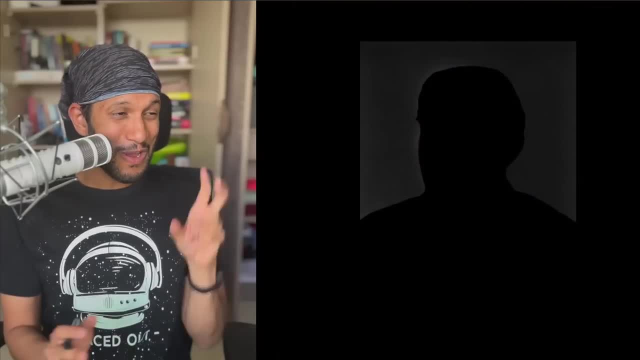 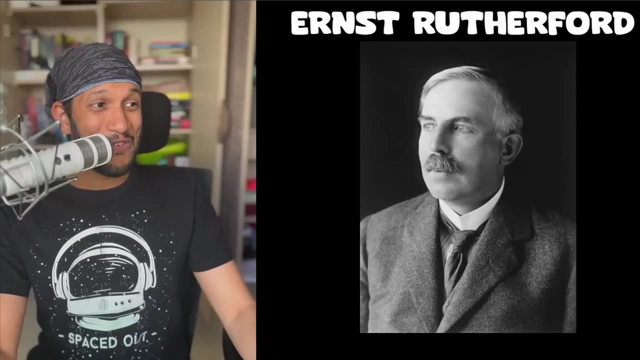 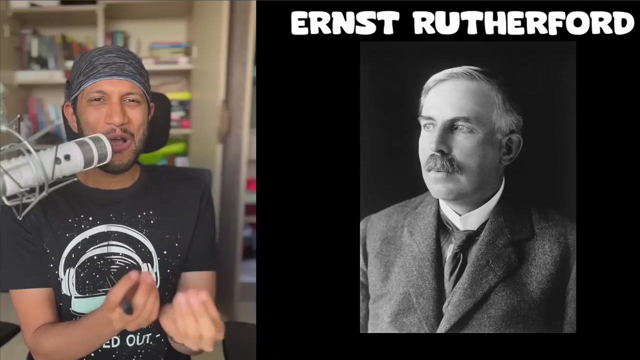 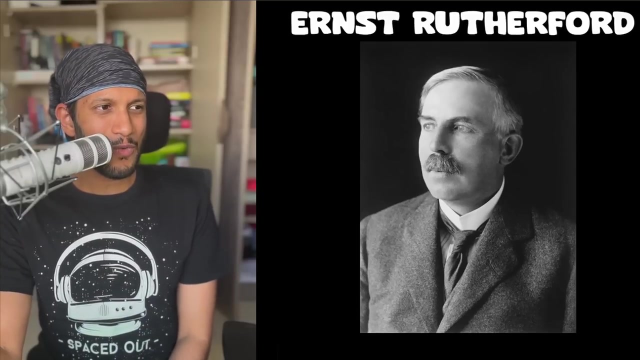 the star of this video? any guesses? it's one of thompson's students himself. that's right, ernst rutherford. rutherford took up the task of testing the plum pudding model. but how do you do that? how do you test what's inside an atom, atom like? how does humanity come up with these things? thompson's idea was quite straightforward. 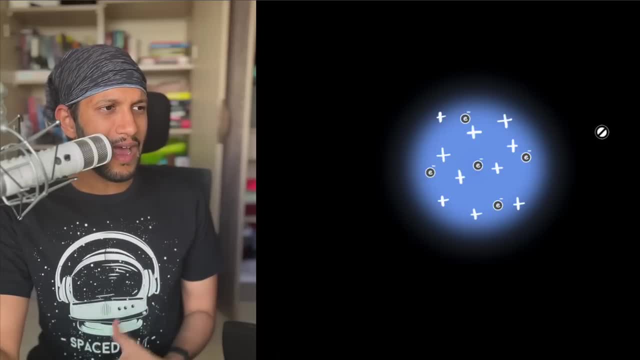 actually thompson said: well, if the entire atom is made of positive charge and there are electrons inside of it, then he started wondering what would happen if you were to sort of like throw a positive charge at it, another positive charge at it. imagine a positive charge, atomic size, bullet. 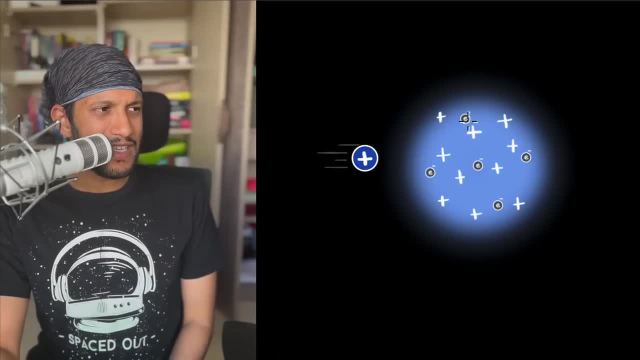 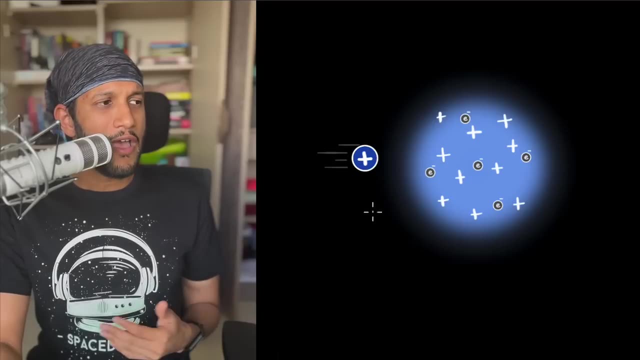 at it. thompson argued that since there is equal amount of positive and negative charge, this particular thing would not experience any force. it wouldn't experience any force when it's outside and, as a result, it'll go straight in and inside as well. it wouldn't experience any force. 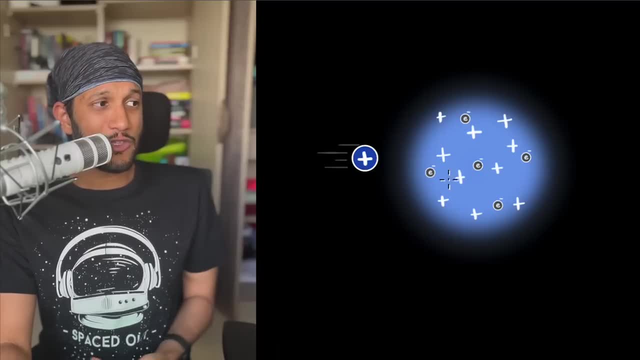 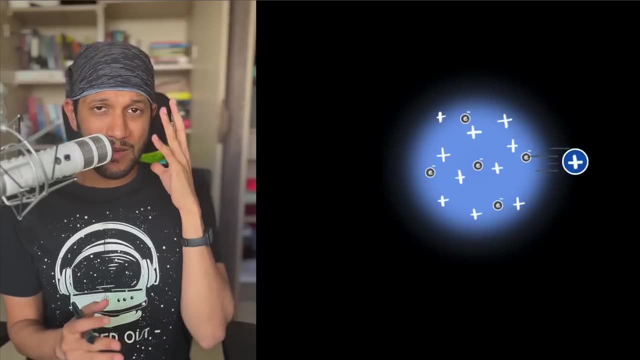 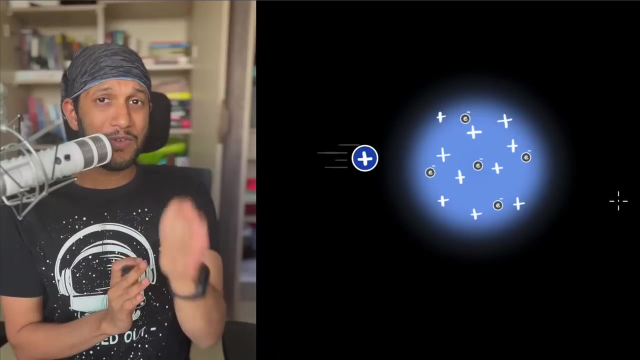 because there's positive and negative charges everywhere, and so that means if i threw a positively charged bullet straight at an atom, it should go straight through. this was the model, this was the idea that rutherford had, and so the idea was: if i can somehow shoot positively charged? 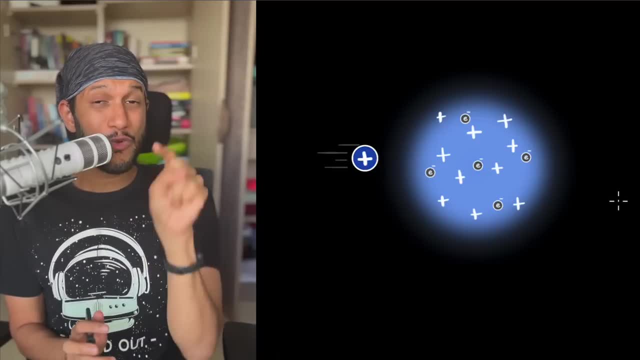 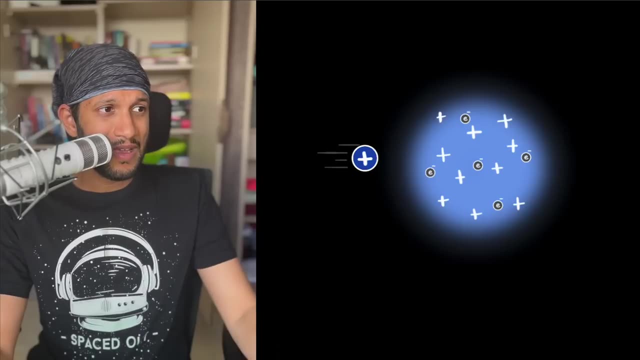 bullets at atoms and if they go through- if i can see that they're going straight through, then i'm done. that is a good test for the plum pudding model. but the question was: how do you do that? this is great in theory, but how exactly do you do this? 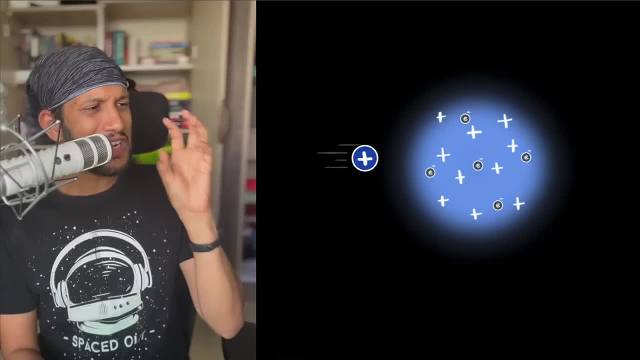 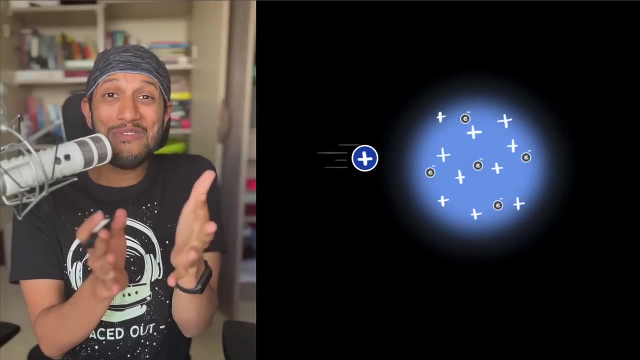 a few challenges. the first challenge is: how do you set your target- atom, like? how do you make sure that you shoot you have one atom target, because most of the stuff that we have is made of billions of atoms? well, rutherford's answer was very simple, and that is that if you shoot a bullet at an atom, 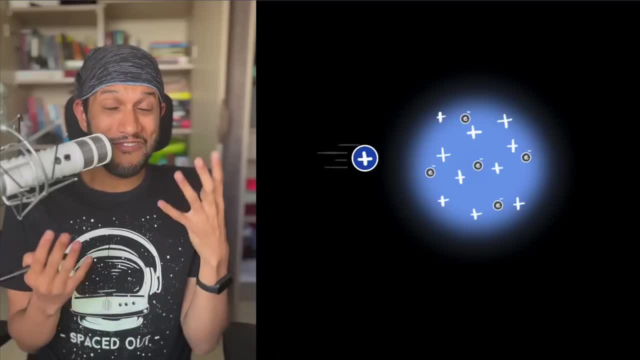 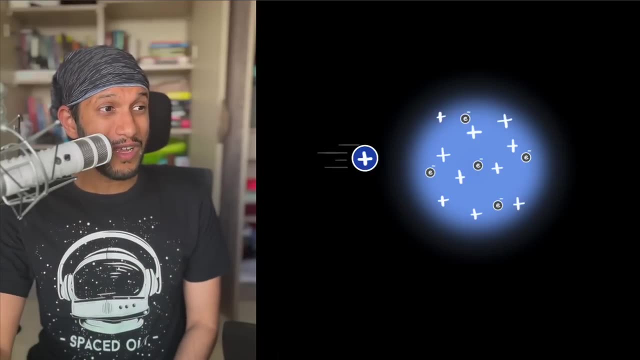 this is going to be a bit difficult for you, because many people assume that it's not going to be as fast and heavy as what you would imagine it to be. but the answer was very simple to him. his answer was: do one shot at a time and that's it. he was about to hit a jackpot. right, he was about to hit a jackpot. 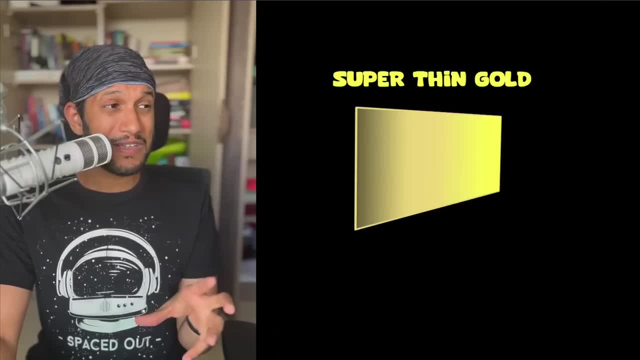 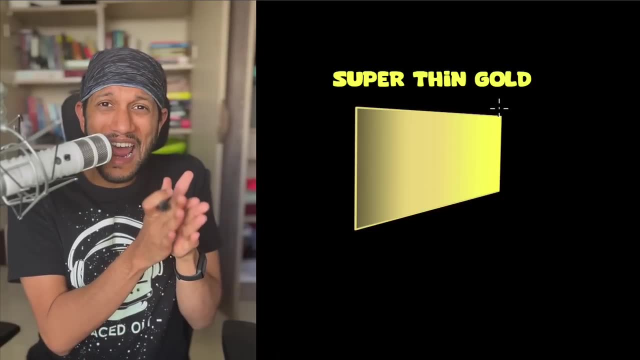 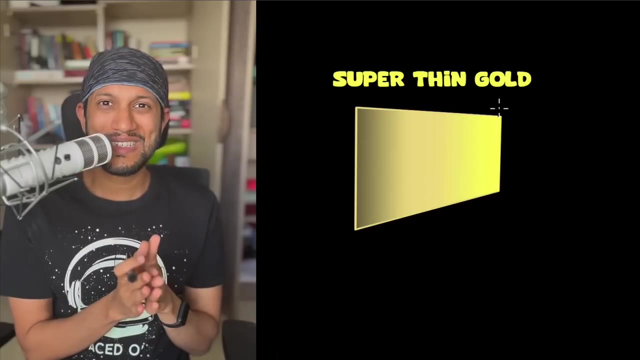 and he actually did it. and there he was about to hit a jackpot and the answer was very simple: let's take a metal. but because metals are very malleable, you can make very, very thin sheets out. few hundred atoms thick, a few hundred atoms. that's super, super thin. for that time at least, 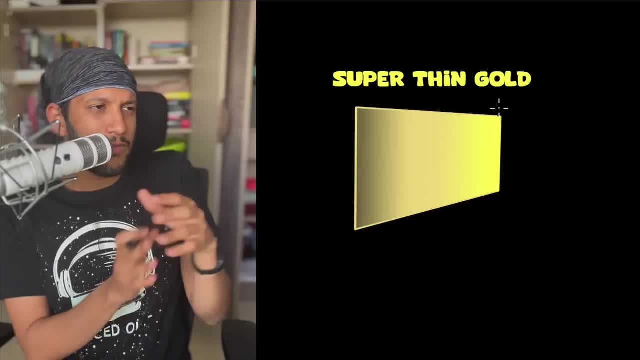 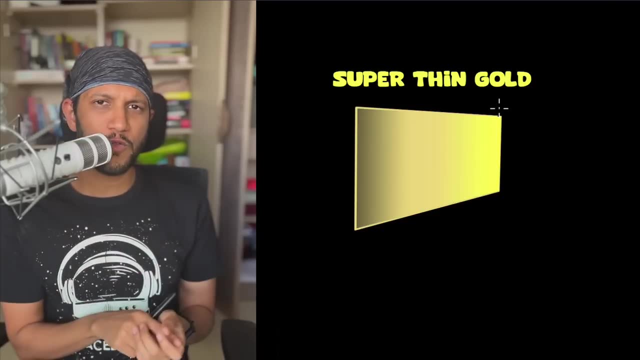 and so, yes, we don't have one atom, we'll have hundreds of atom, but that's still fine. the idea is that if they don't exert any force, the positive charge bullet should just go through. maybe because there are hundreds of atoms, it might have some small deviations, but that's still okay. 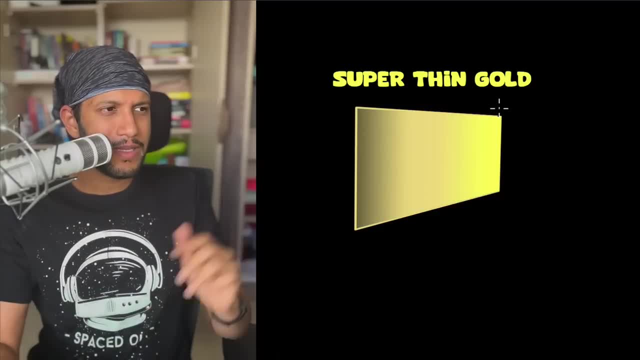 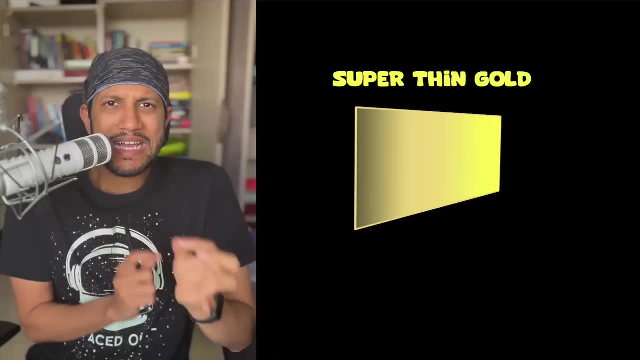 but most of it, mostly, it should go just straight through. that's the whole idea behind the plum pudding model. okay, we have one challenge done, we have the gold foil. the next challenge was: how do we detect that the particles have gone straight through or not? how do we detect the path? 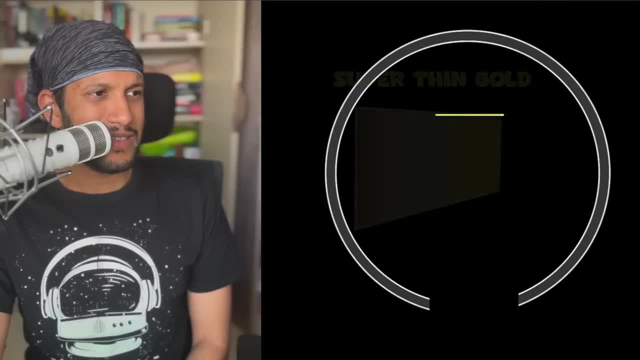 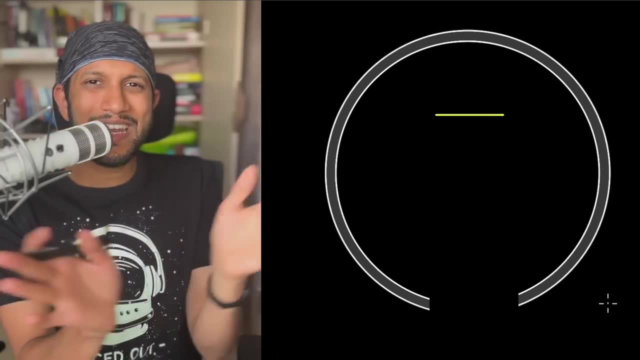 well, for that. rutherford's idea was to construct an apparatus like this where you have a thin- this is the thin- gold foil. you're looking at it from the top now and the whole thing was like a stadium. you have like a stadium boundary over there, and it was. 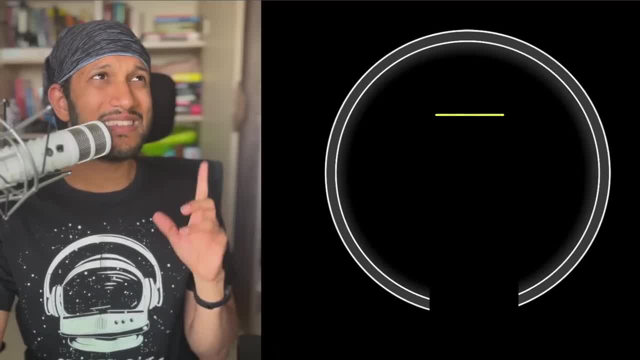 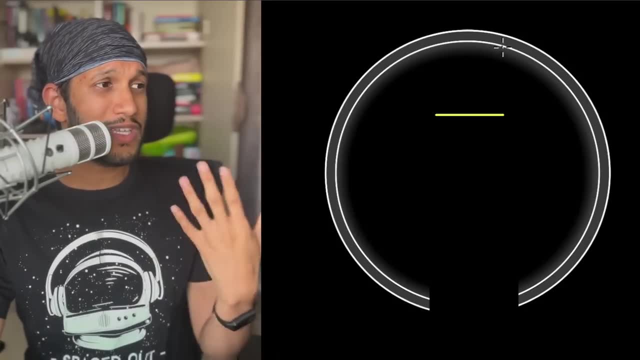 coated with some kind of a chemical. i forget what that chemical is. i think it's zinc sulfide or something. the property of that chemical is, when a positive charge- or you know positive charges- goes and hits it at that particular spot, you would get a glow. so, for example, if you see a glow somewhere over here, 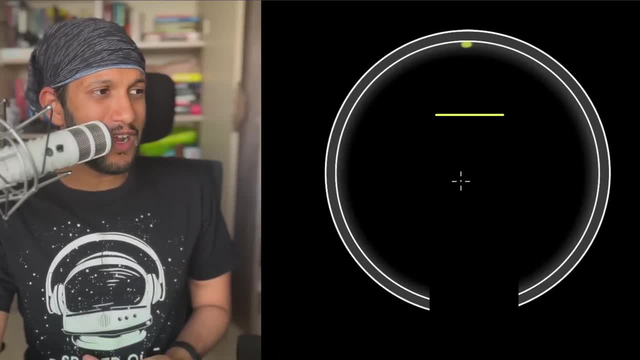 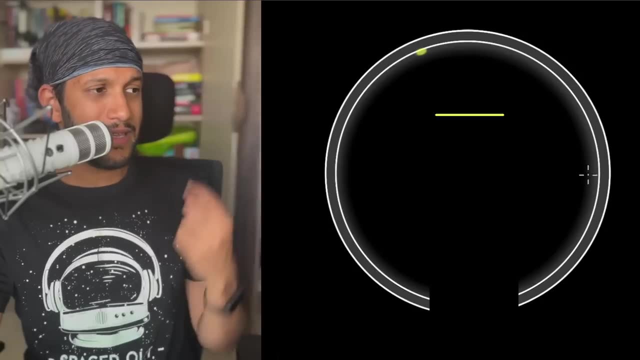 that means that that particular bullet, if it's shot from here, it must have gone through like this and landed over there. on the other hand, if you see a glow somewhere over here, then we can see that if it was shot from here, it must have hit over here. it must have gone like this, so you. 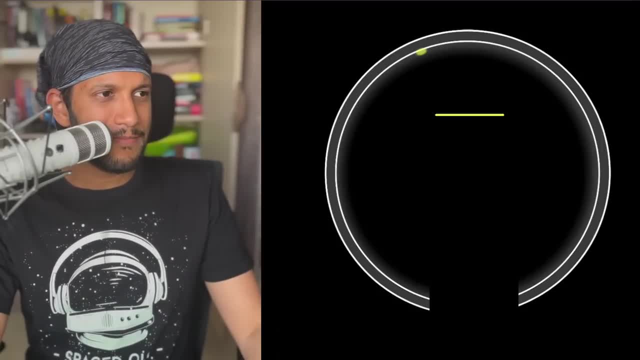 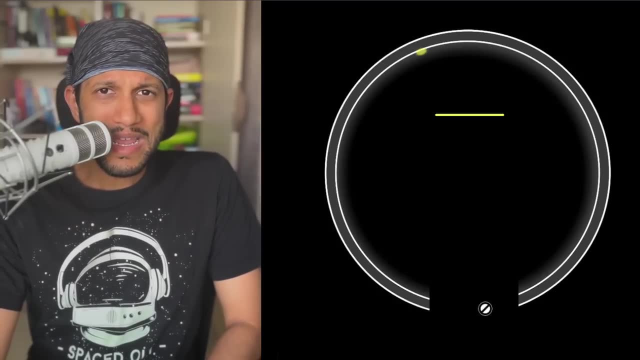 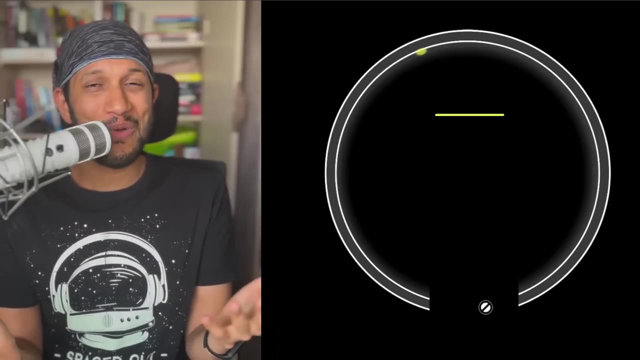 can sort of think about the path over there. all right, no need to junk you, we'll have a whole page that we'll cover in our next video. just a tiny little question at the end: camera dynamic. so that was done. that was that. but the last question we might have on the four is: 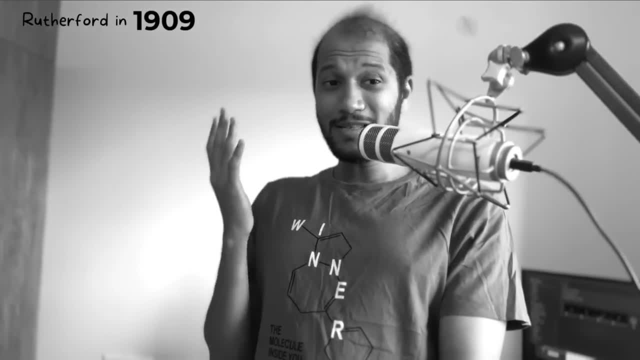 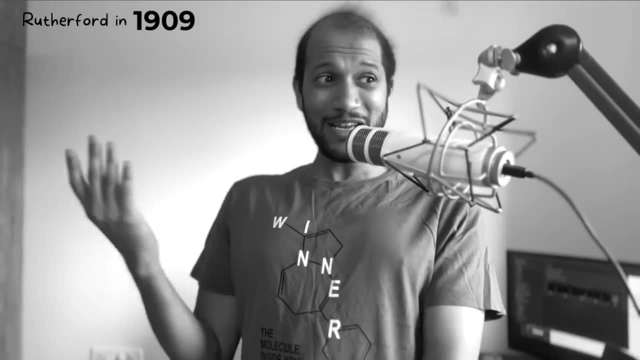 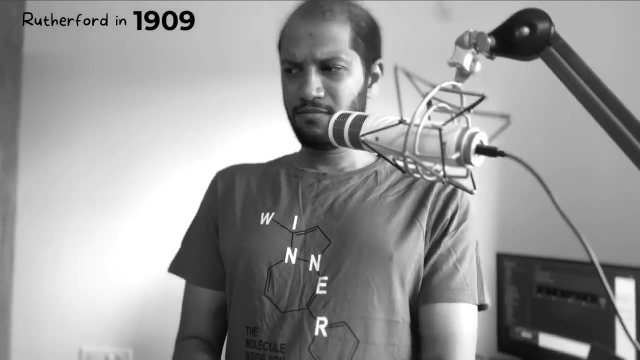 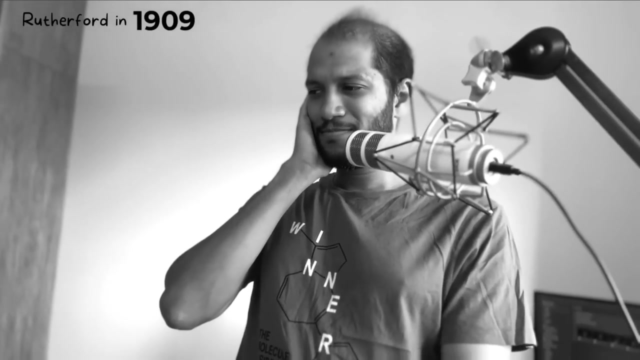 where do we get positively charged atomic bullets? where does the other four find that from it's 1909? there is no technology over here? i don't know why i even signed up for this. oh my god, wait, why is curie calling me? hey, curie, what's up, brother, for just wanted to call you to. 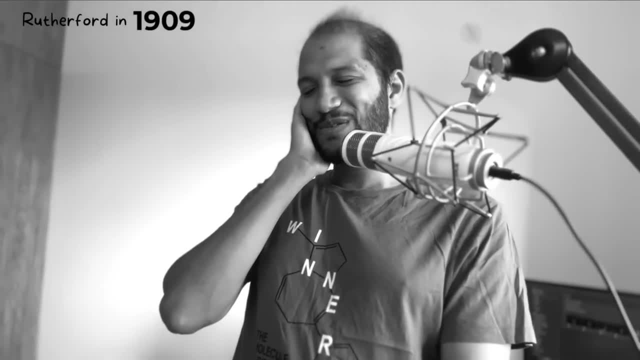 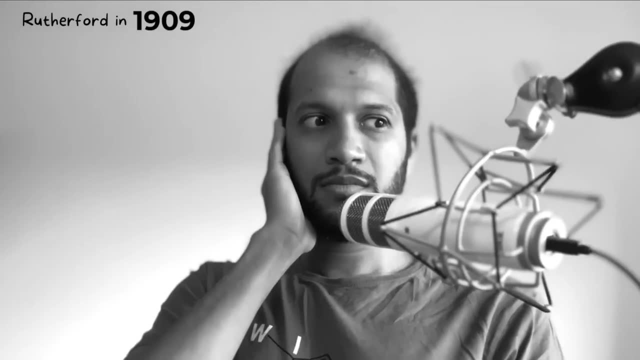 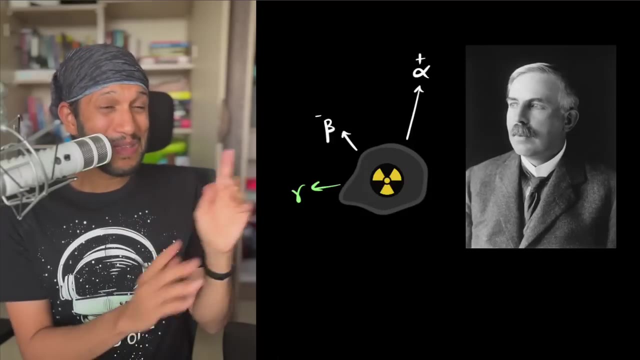 congratulate you again for your noble prize in chemistry last year. you know the one where you worked on the alpha particles, which are like positively charged bullets coming out of radioactive substances, curie. i gotta call you back, that's right, rather, for i had already gotten a nobel prize the previous year in chemistry for his groundbreaking work on radioactivity. in fact, 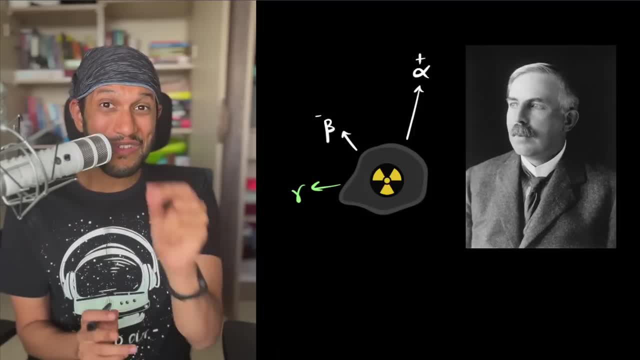 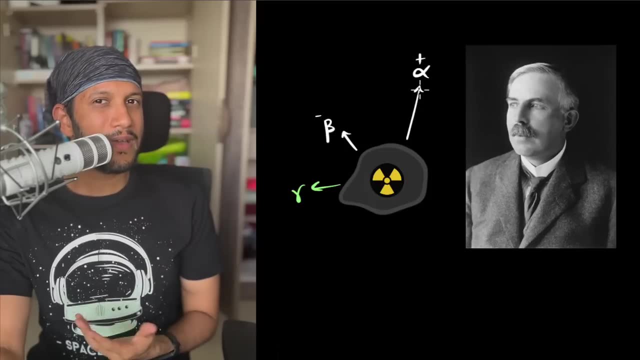 he did a lot of research in figuring out what the alpha particles were and he had figured out that the alpha particles are positively charged bullets. today we know that alpha particles are basically helium nuclei and beta particles are actually electrons and gamma is basically photons. but back then what was important? 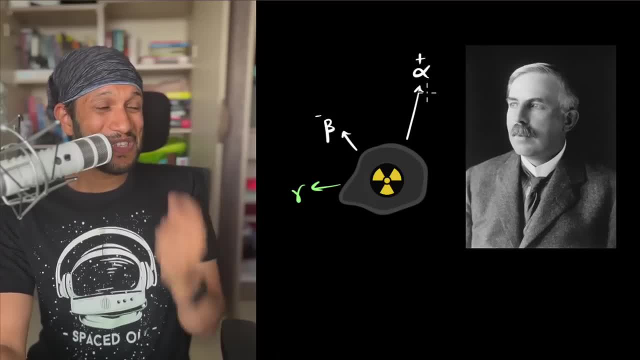 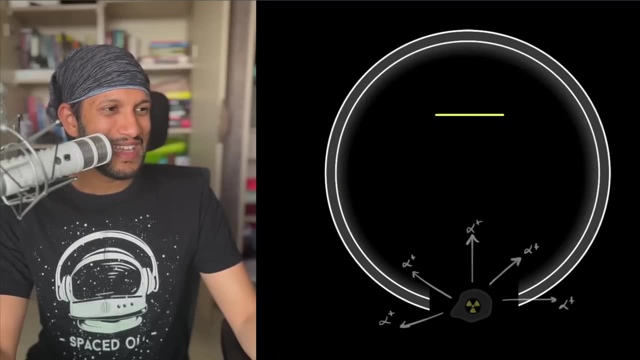 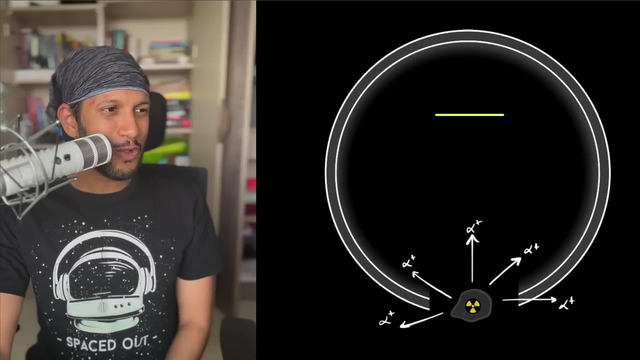 is that they knew that alpha particle was positively charged. and so what? what would rather for do now? all rather for had to do was use his some kind of a radium isotope, which is which is the source of an alpha particle, and of course, enclose that so that you have more. 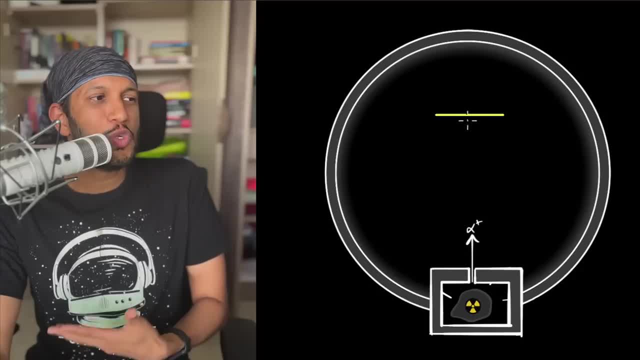 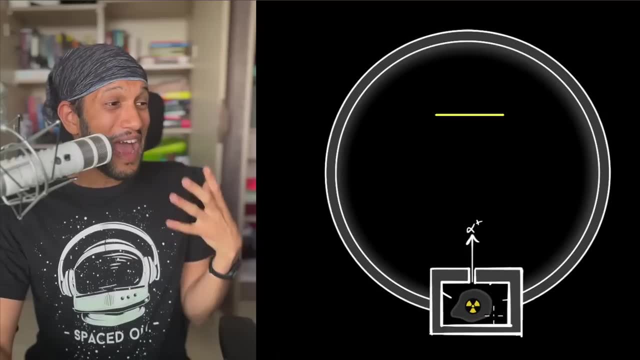 control over the direction. you only want the alpha particles that are coming towards the gold foil, and that's the last piece of the puzzle. so we now have everything. we have the gold foil, we have the alpha source, we have the alpha particle source, we have zinc sulfide all around. so we know. 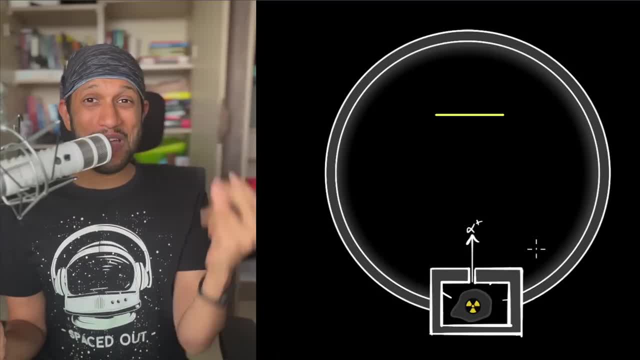 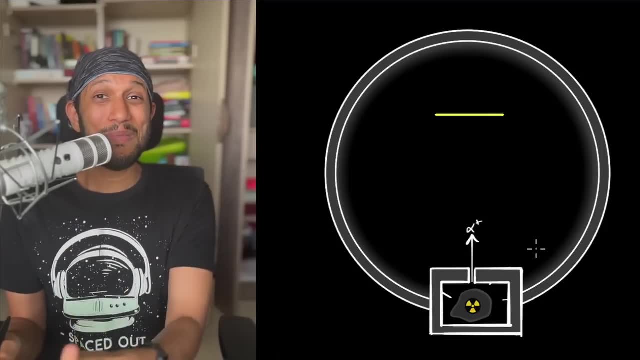 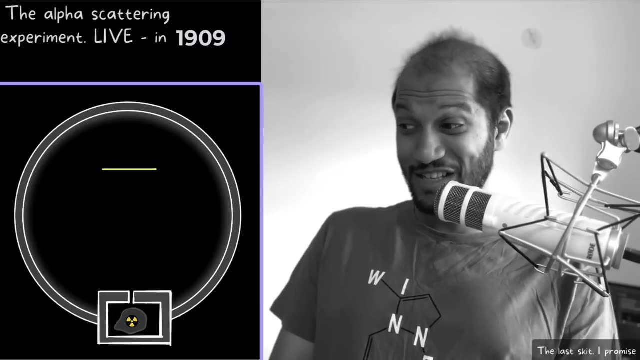 where these alpha particles land. all we have to do is do that experiment now and once again, let's go back in time one last time and look at this experiment. done, live. all right, folks, are we all ready? we have everything set up. we also have our predictions. everything is supposed to go straight. 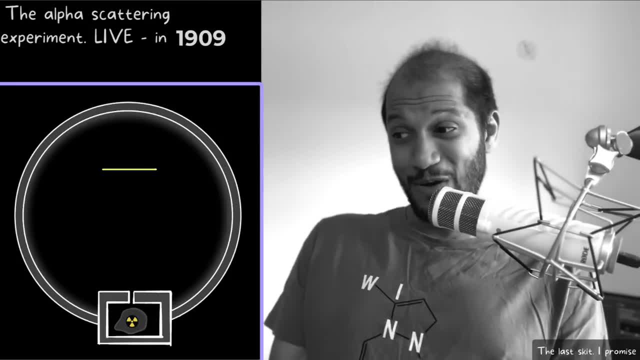 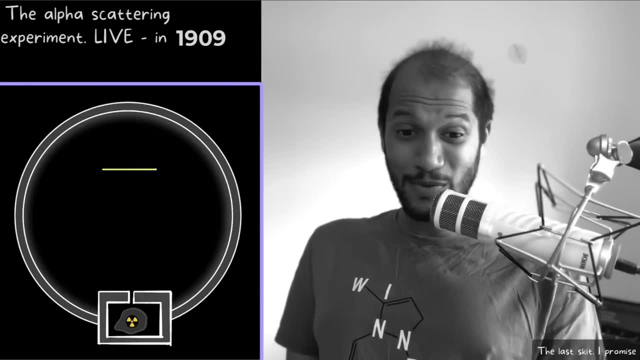 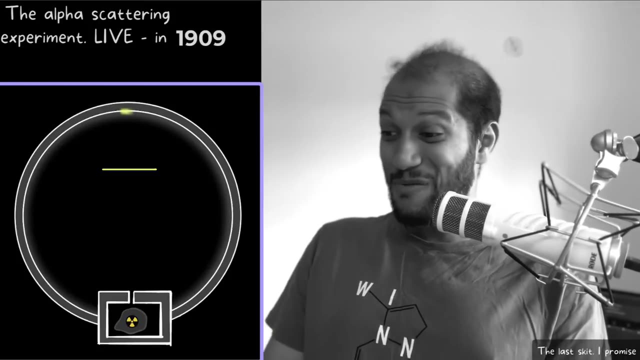 through and that's obviously what's going to happen, because you know, thumb pudding model is awesome, jj, thumb son is awesome. it's obviously right, everything is just right. i have thompson on the speed dial as well, because we know we're going to confirm it. okay, ready, let us start there we go, there we go. 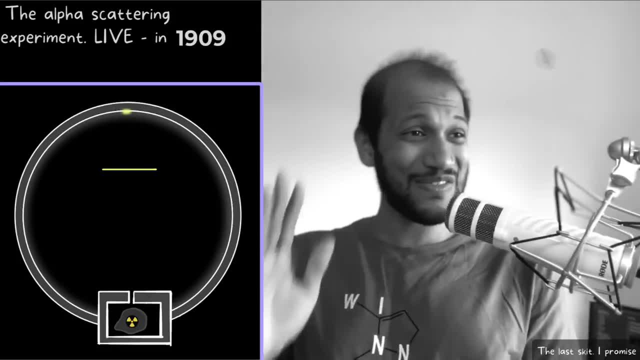 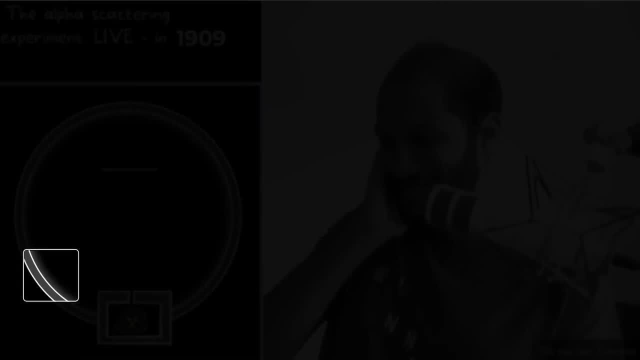 all the alpha particles are going straight through. awesome, high fives, high fives. should i call thompson now? i think we should right, like, i mean, it's happening, it's happening. all right, let me call him. hey brother, what's up? wait, did you see that i'm gonna call you back? yeah, yeah. 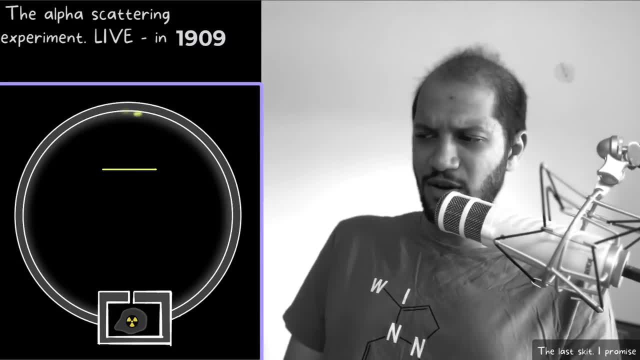 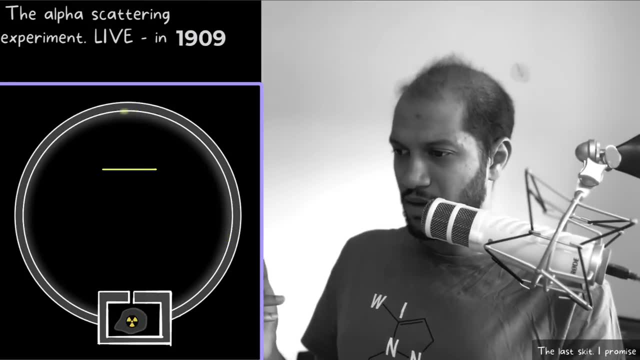 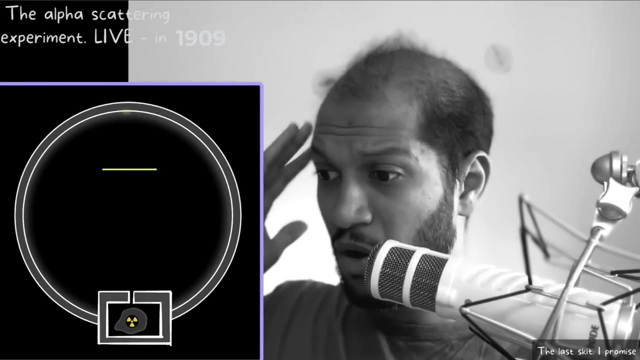 it's just a glitch. it's just a glitch, it's fine, it's, it's fine. i think it's it's not not a big deal. wait, there's another one. what's happening? wait, there's another one, and there's one more. wait, this, this, this can't be no, no, this can't be no, no. 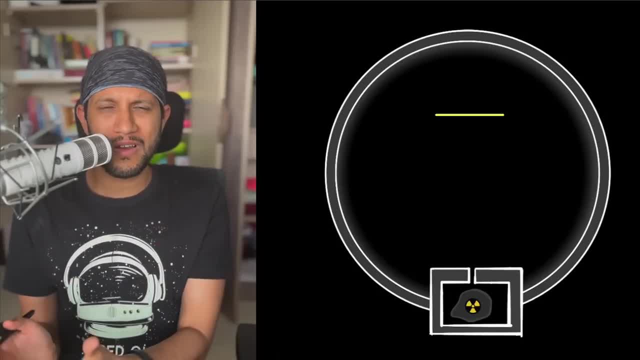 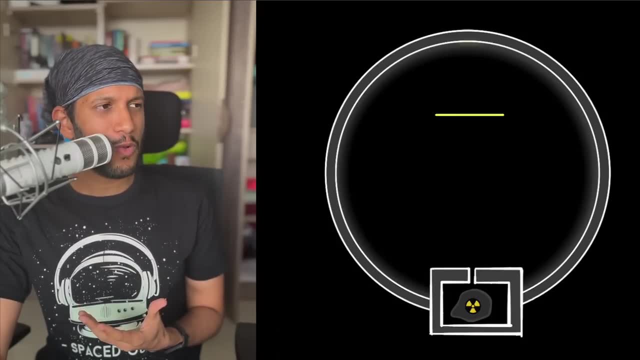 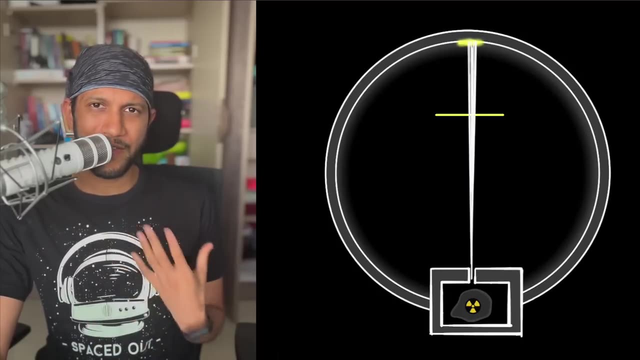 what just happened. why was rutherford's so shocked? well, if you go back to the experiment, we saw that most of the glow was right behind the goldfoil and this was the one that we predicted. this basically meant all the alpha particles over there went straight through. but if you watched that, we were that part, that clip carefully. 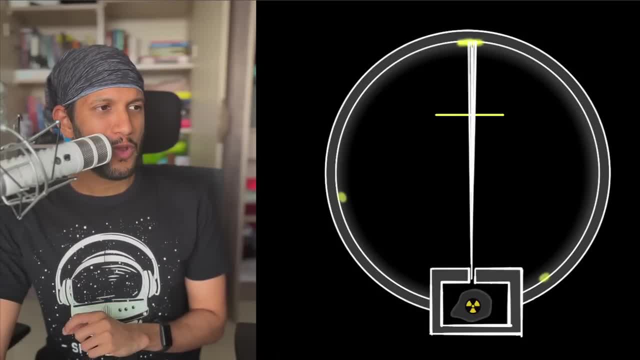 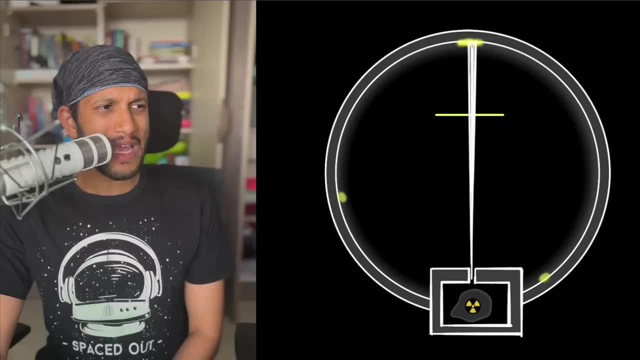 we also found some glow, which was behind. this was the one that shocked rutherford and his friends, because that meant that alpha particles are bound up behind the goldfoil. and this was the one that shocked rutherford and his friends, because that meant that alpha particles are bound up behind the read pathway. so that's a good problem. 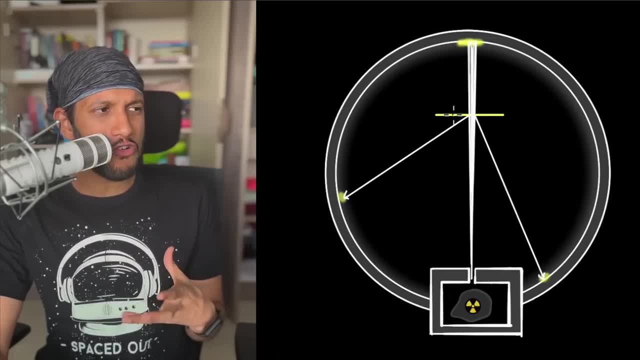 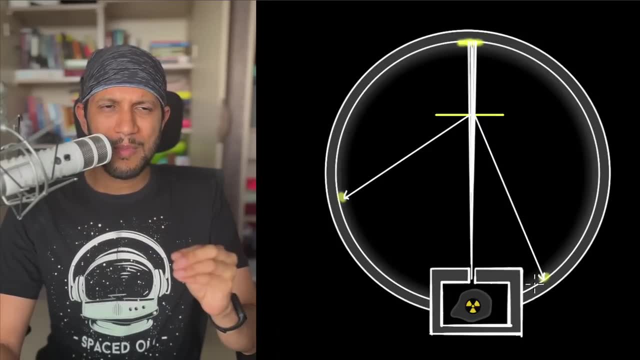 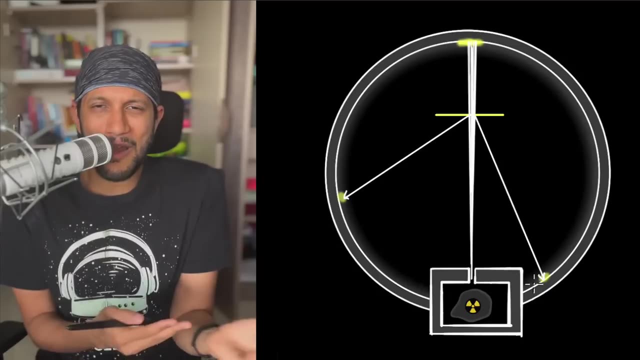 that alpha particles are bouncing off of gold atoms. but you may ask: well, Mahesh, why is that such a huge deal? because, as a scientist, you probably know that experiments don't always give you the exact same observations. right, because that's, that's part and parcel of science. 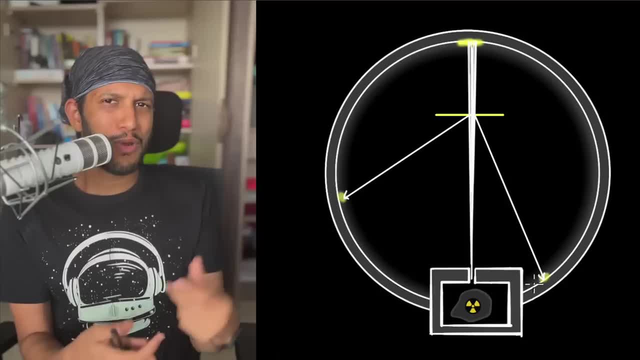 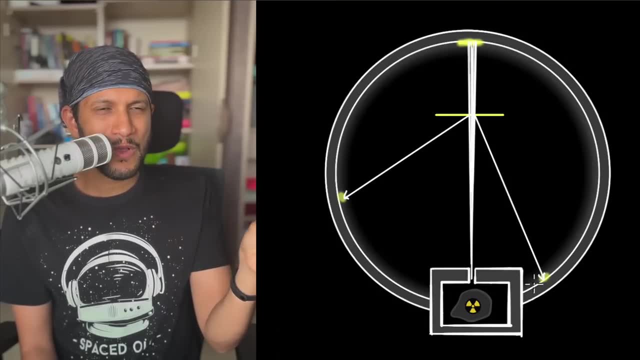 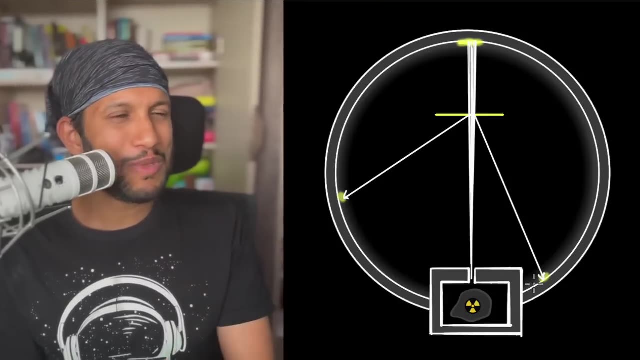 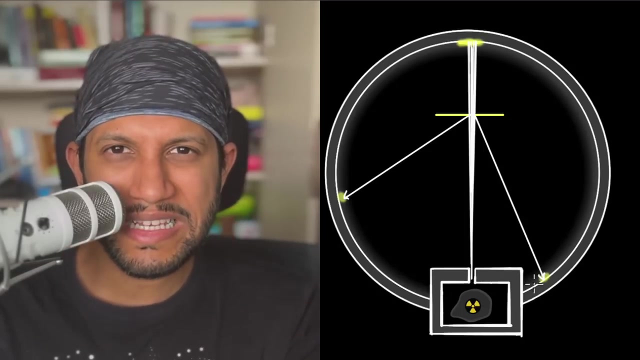 and so maybe something like that has happened over here. we just need to tweak our model a little bit, right? no, what this meant, which we'll understand now, something dramatic. this meant that the plum pudding model had to be completely discarded, not tweaked, not changed a little bit completely. 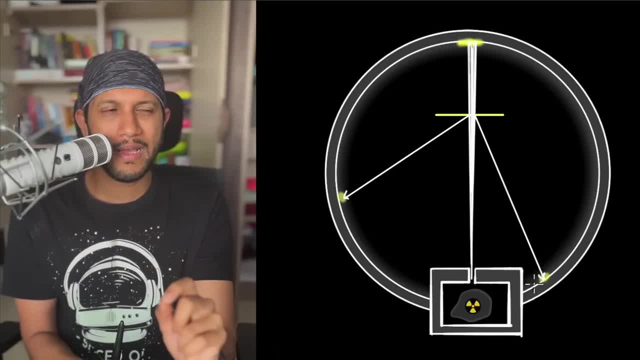 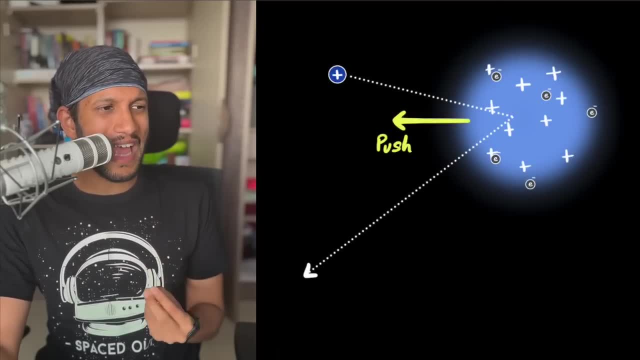 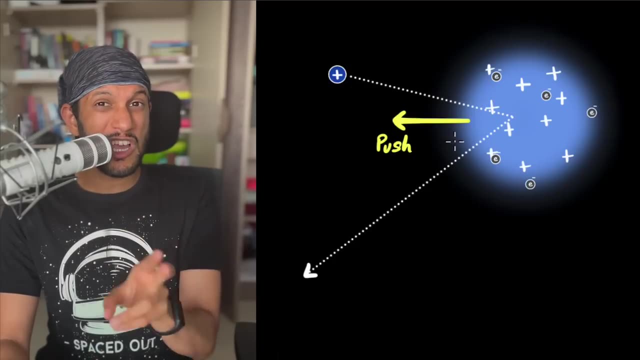 discarded, why? well, let's look at it. if the alpha particles are bouncing off like this, there must be a signal, significant force acting on them, and since alpha particles were known to be pretty energetic, this force needs to be pretty high. the big question was: where is this force coming from? 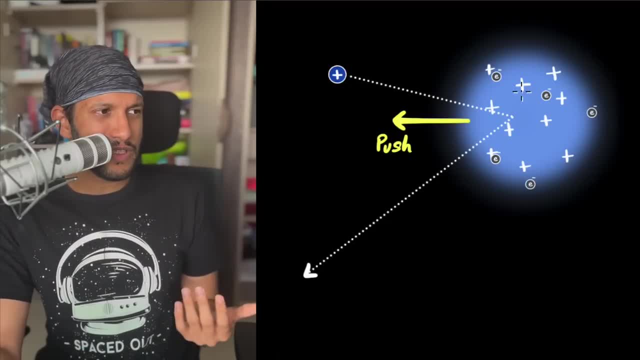 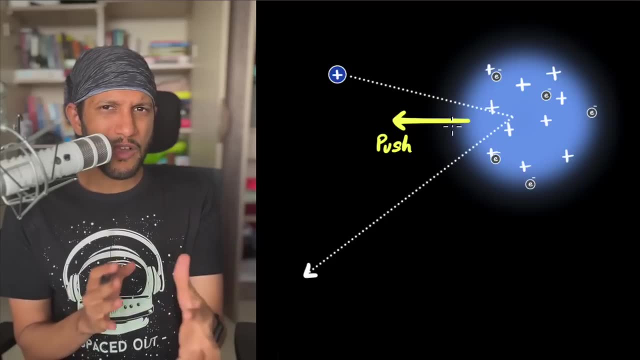 we already saw that because the according to the plum pudding model, because everything is pretty neutral, there's no way the plum pudding model can generate that much force. and Rutherford did some back of the envelope calculation. even if you have hundreds of atoms and even if it's not. 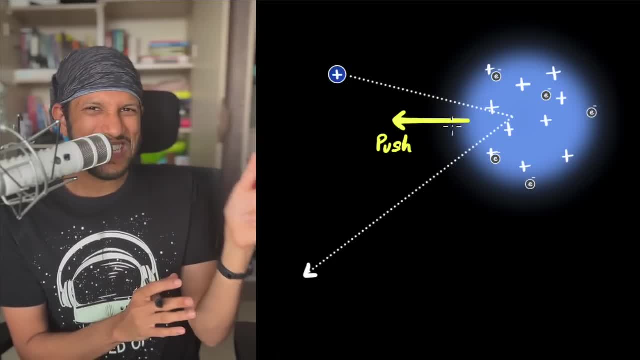 perfectly distributed. he saw that the force needed to create that much force, and so he did some back of the envelope calculation. and he saw that the force needed to create that much force, and so he did some back of the envelope calculation. even if you have hundreds of atoms and even if it's not perfectly distributed, he saw that the force needed to create. 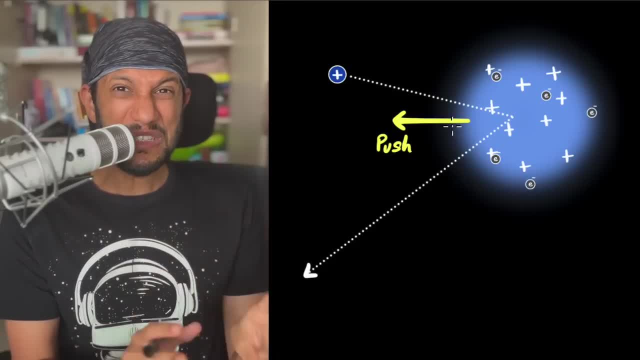 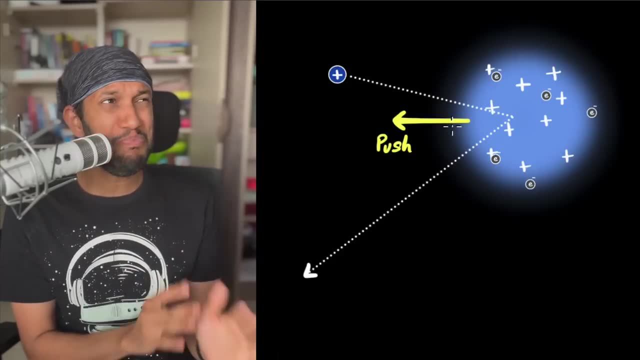 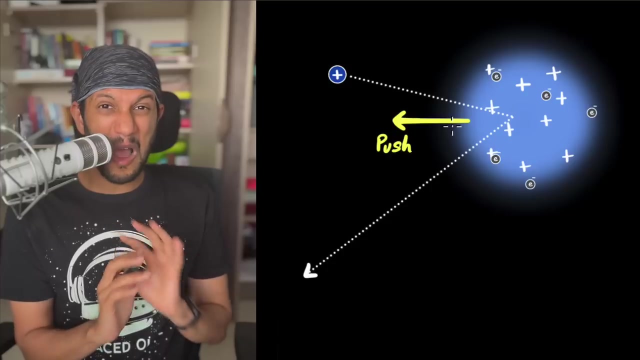 that kind of a bouncing off effect is billions of times stronger than what the plum pudding model can ever give you. billions of times stronger. that's not just a small error, that's a huge error and that's why Rutherford was shocked and he was trying to figure this out for another. 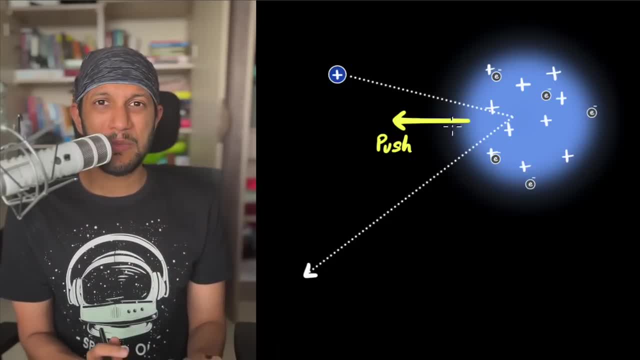 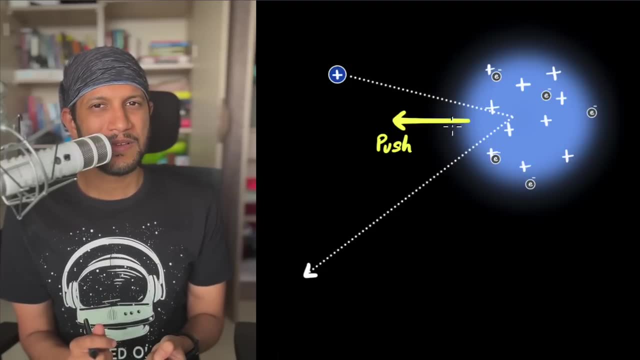 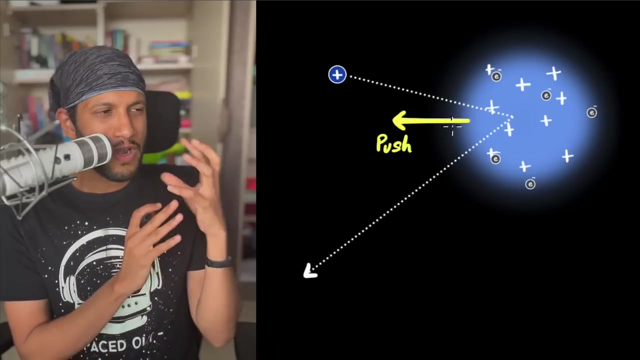 couple of years by doing multiple experiments and trying to figure out. what does it all mean? and eventually he did figure it out. he realized that he had to throw the plum pudding model out of the window and just start from scratch, and so what he realized was that 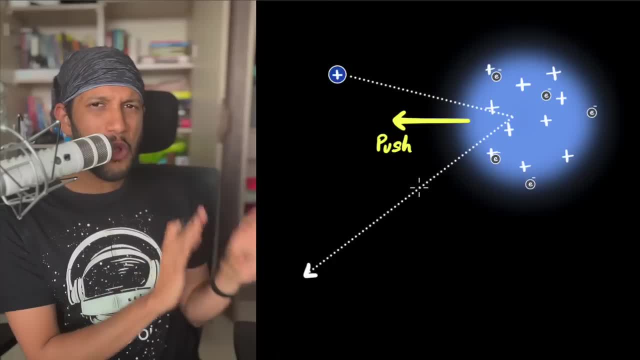 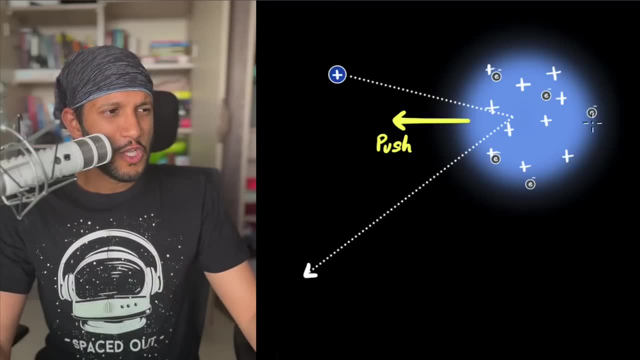 if i need to generate that much force. there is no way that the positive charge can be distributed uniformly throughout the atom. that's just not possible. so he just he realized the only way that the alpha particles can get that much force, and that's why Rutherford was shocked and he was 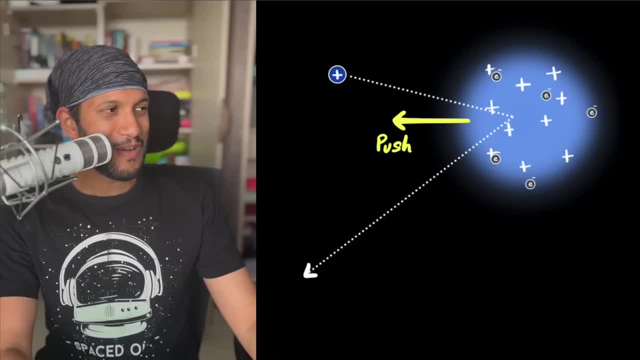 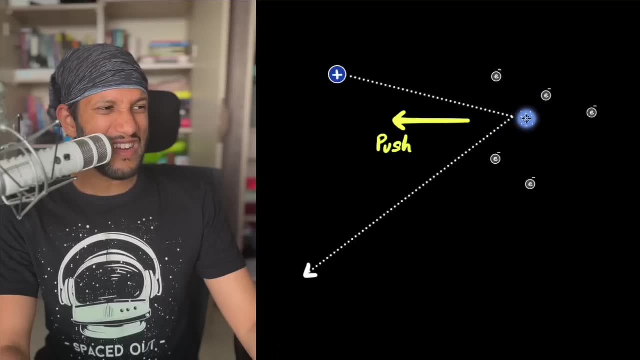 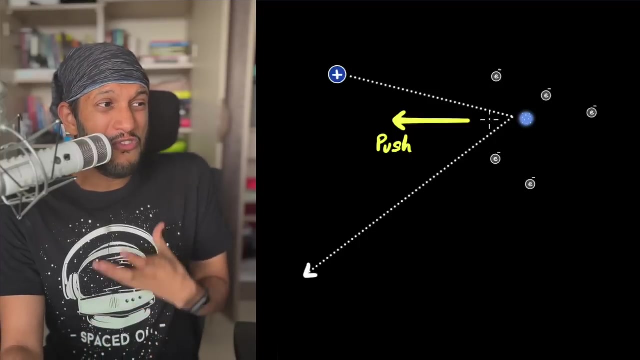 going to use Ruther's Mohr mol County theory including example. the positive charge is not distributed throughout the atom. but if it was concentrated in a very tiny space at the center of the atom? because then, look, the alpha particles can come very close to that positive charge and from coulomb's law you probably know, the closer 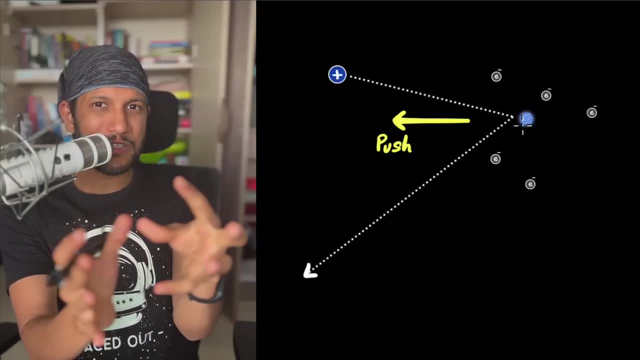 something can come. the closer charges are, the bigger the coulomb repulsion, and so you can have a very strong coulomb repulsion and you then get this block because it's economies of verse. and so we're going to go with a hashing like over this: soyль, reduced mass, everything as a Ukulele. so if you push, 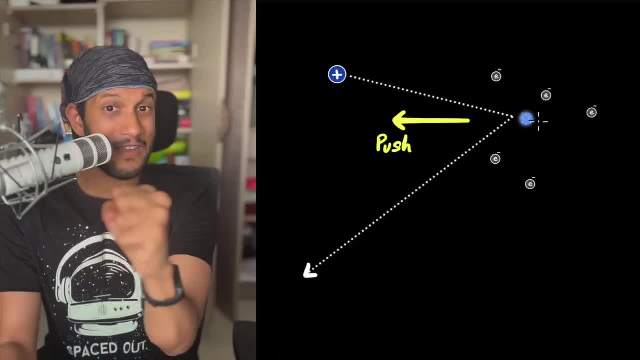 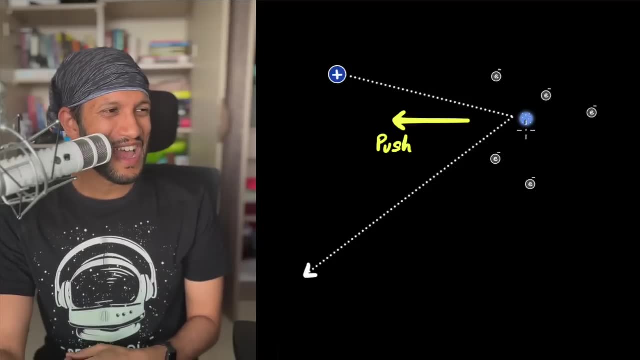 if, and only if, that all the positive charge is concentrated at the center. no electrons over there. so you feel the full brunt, the full grunt, full brunt, full brunt of the positive charge. and there, therefore, he said that all the positive charge must be concentrated at the center and he called: 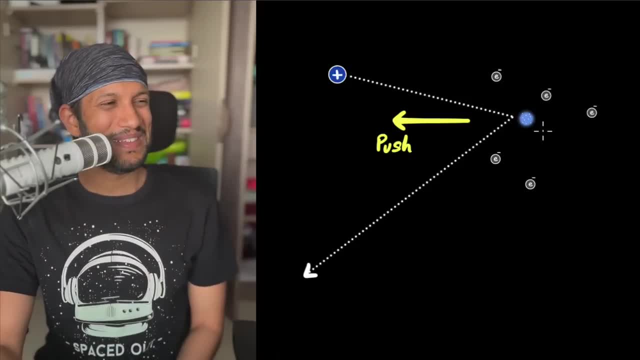 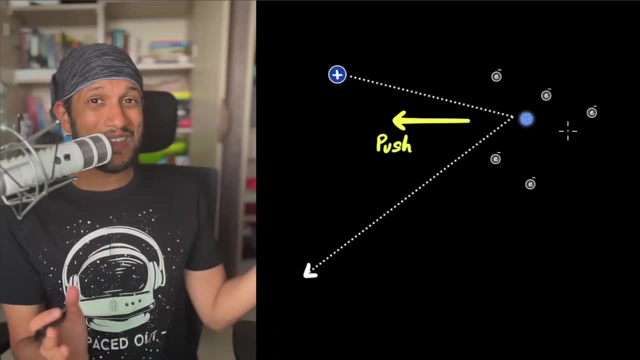 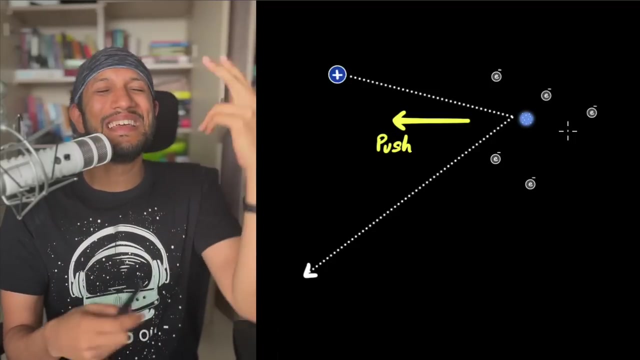 it, the atomic nucleus, which you're probably familiar with. and what about the electrons? well, you probably know how the story goes now. he compared with our planetary model. he realized that, just like how the sun pulls all the, what sun pulls all the, what do you call that? planets? 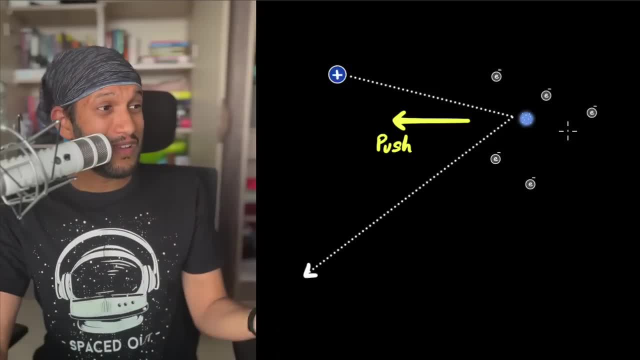 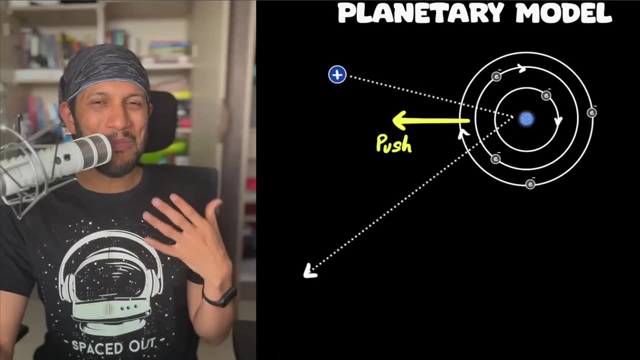 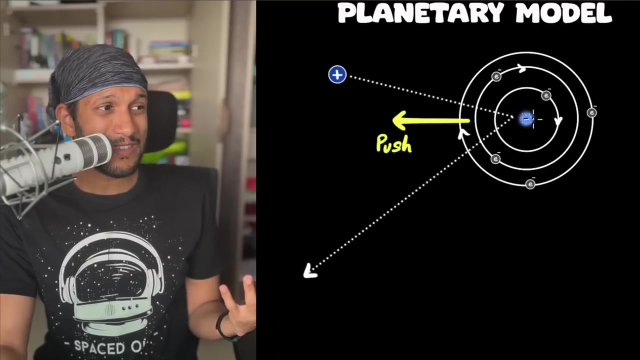 sun pulls all the planets and makes it go around it. similarly, this positive charge will pull all the electrons and make them go around it and the planetary model was born. and this perfectly fit the data because, look, because the thing is in the center. most of the times the alpha particles will. 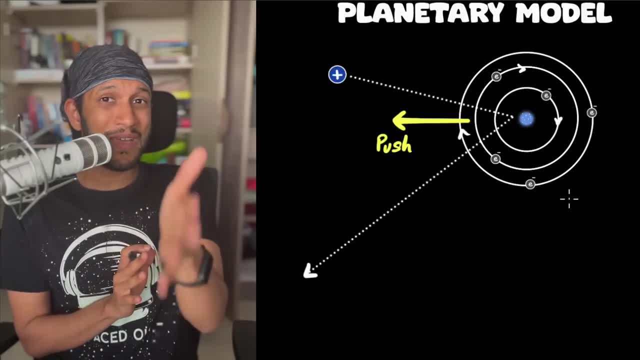 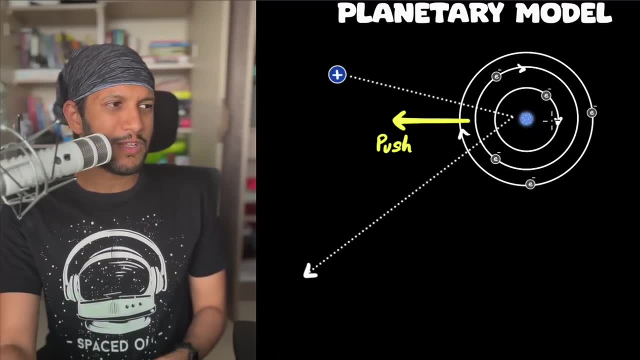 not even come close to it and therefore they'll go you through, and that explained why, most of the times, we did see alpha particles going straight through, and then, sometimes- about 1 in 20,000- we found that the alpha particles were scattered by a very large angle, and so this alpha scattering experiment, as we call it today, is the one 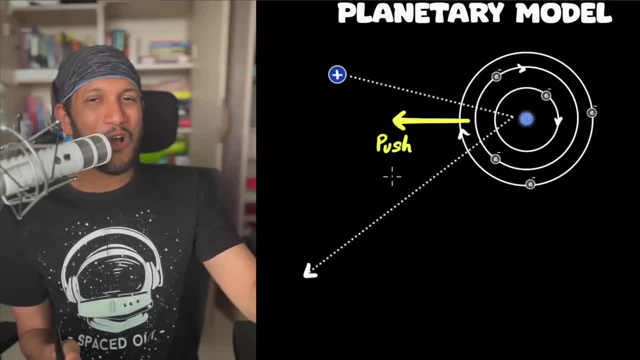 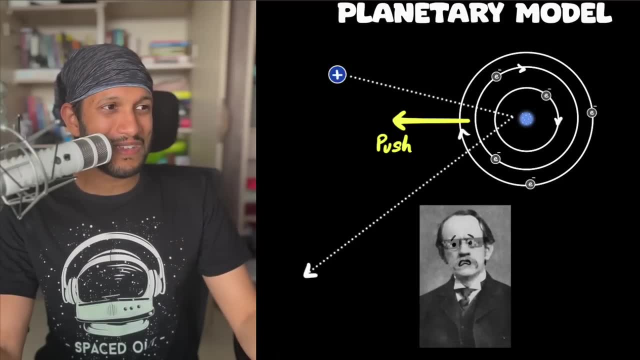 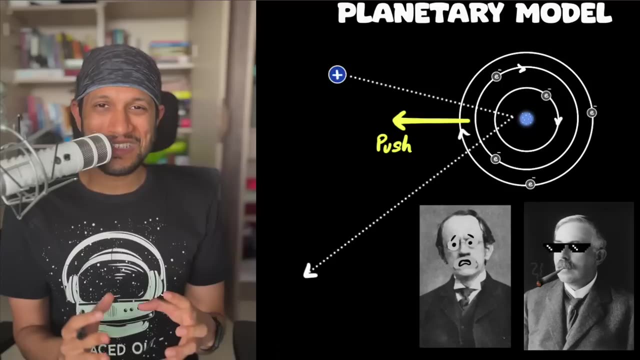 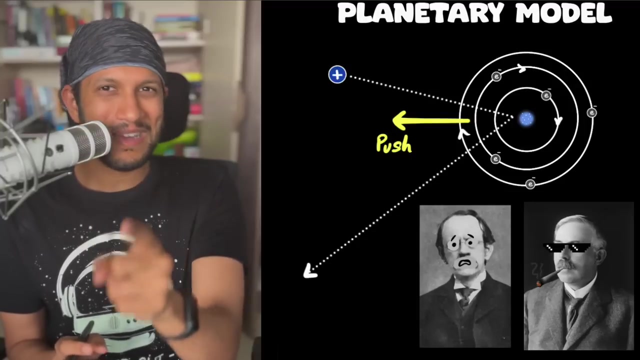 that led to the 1911 discovery of the planetary model and the atomic nucleus. so the plum pudding model was discarded, poor Thompson, and the planetary model was born. the student had become the master. but now comes the shocking consequence part. it was not a clickbait. what is the shocking? 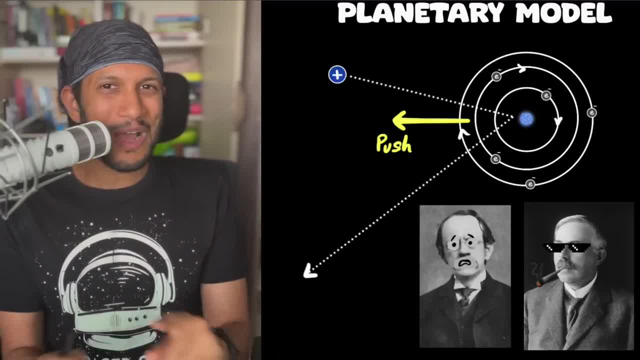 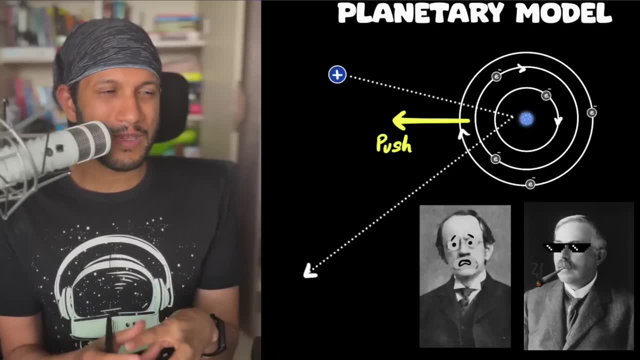 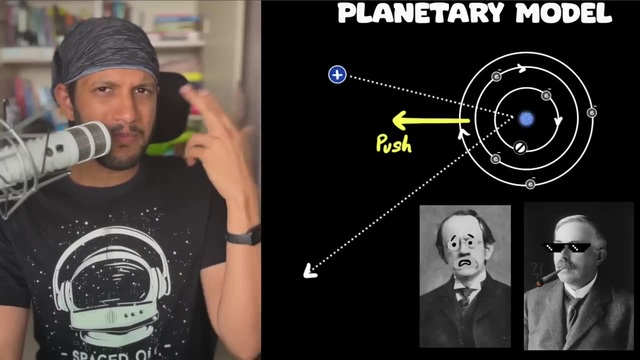 consequence of this that is not discussed in our textbooks, and how is it related to what I initially talked about at the beginning of the video? well, Rutherford was able to do a back of the envelope calculation, based on just Coulomb's law, how small this nucleus needs to be. and you can, you can see that right if the nucleus is too big. 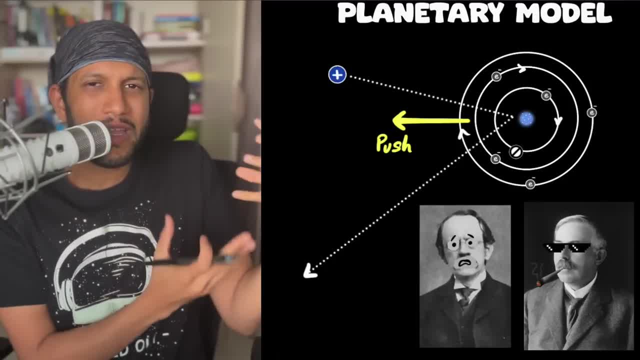 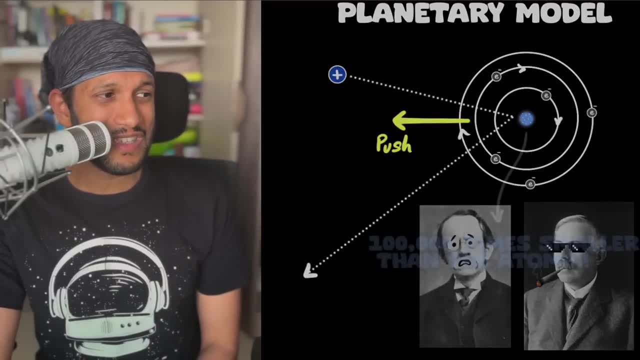 it'll not be able to come very close and you'll not be able to generate the force. just by looking at how much force he got, he was able to figure this out and his back of the envelope calculation showed that the nucleus needs to be at least a hundred thousand times smaller. 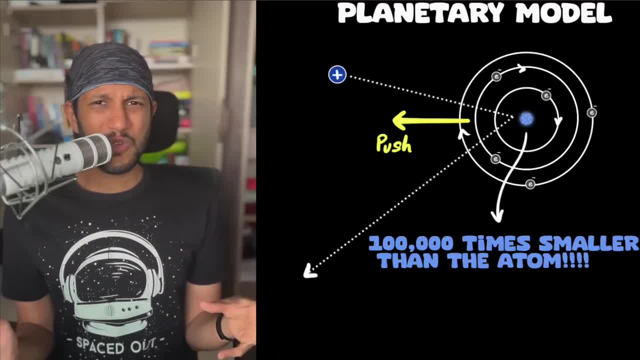 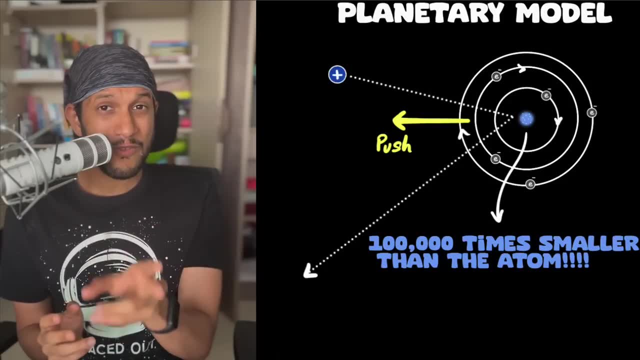 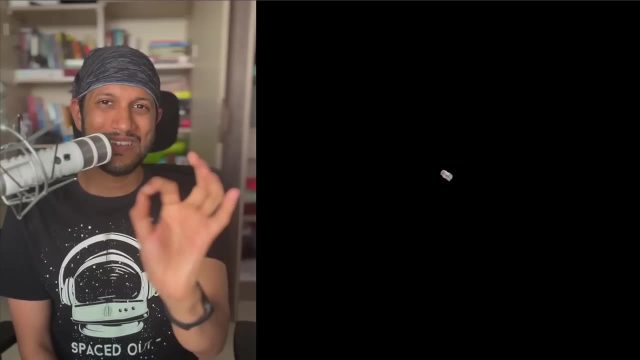 than the atom. and why was this so shocking, you ask? well, first of all, my brain cannot understand these large numbers. 100,000 is too big for me. so what I should, what we'll do, is we'll scale it up. imagine: the atomic nucleus is the size of a grain of sand by that. 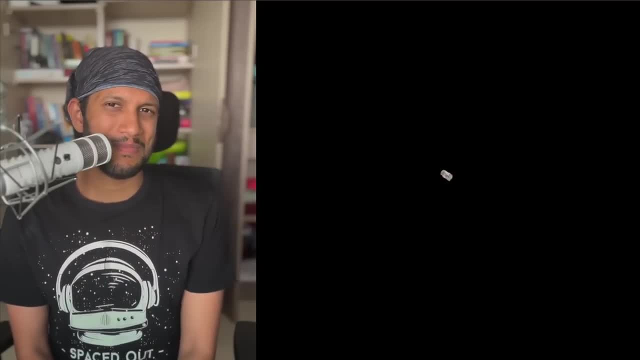 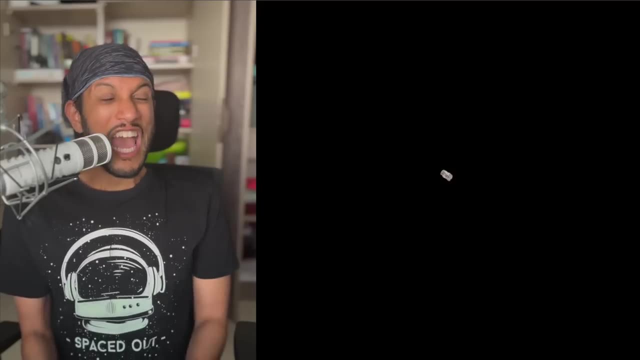 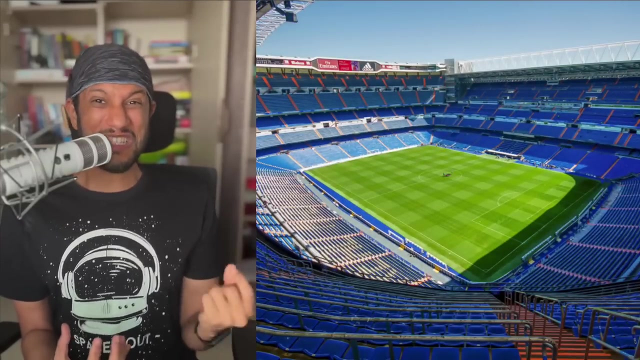 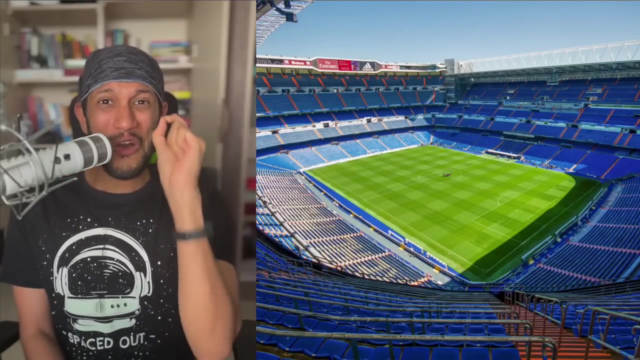 scale. what would the atom look like? what would the atom be? just pause and think about? will it be a lemon? will be a basketball? it would be a freaking cricket stadium. that's how small the atomic nucleus is: the entire cricket stadium. if you consider it to be the atom, the nucleus is a grain of sand. 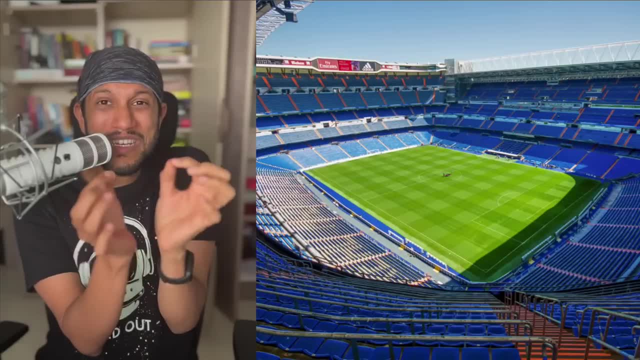 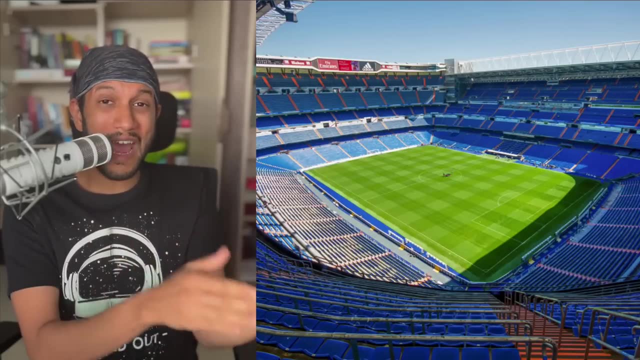 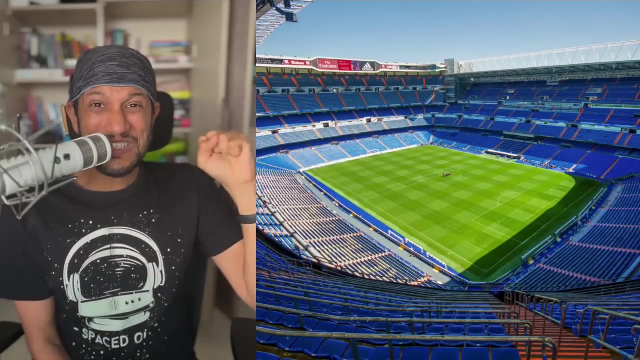 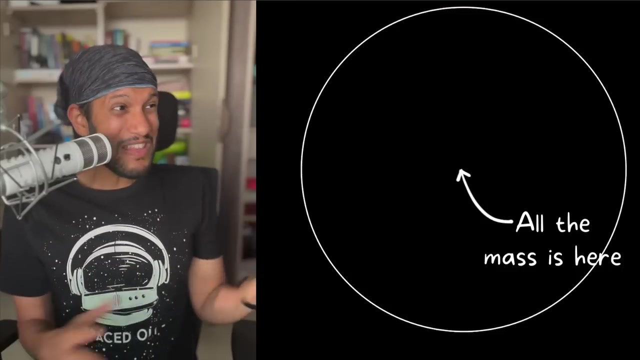 and we already saw that electrons are incredibly tiny, incredibly mass. less part they have mass, but their mass they are very light particles. this means all the mass of the atom is mostly in the positive charge and now all the mass of the atom is concentrated in that tiny space, making the rest of the atom empty. think. 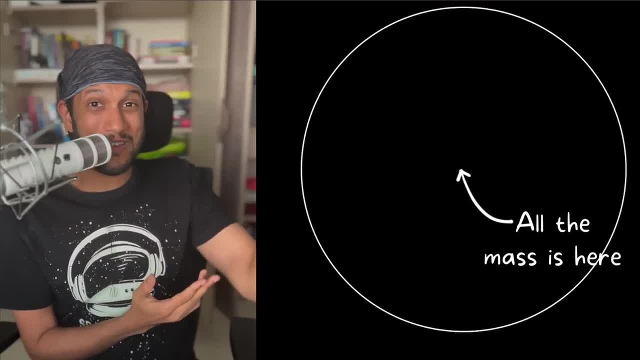 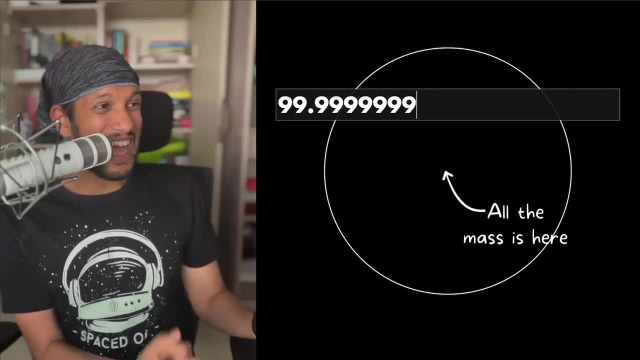 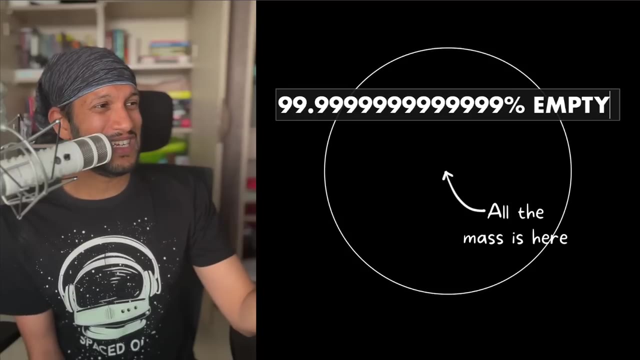 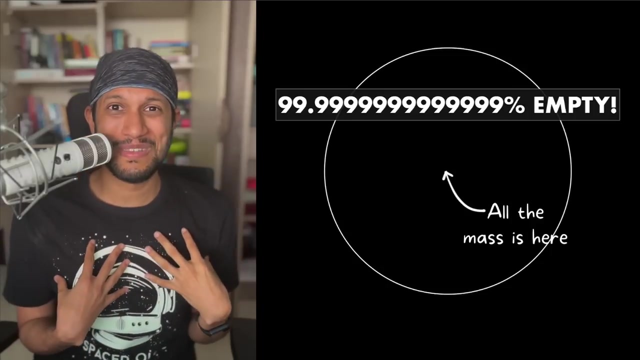 about how empty that atom is. if you actually put it to numbers, you'll find our atom is 99.999999999999% empty. all atoms are this much empty. we're made of atoms, which means I am this much empty, you are that much empty. 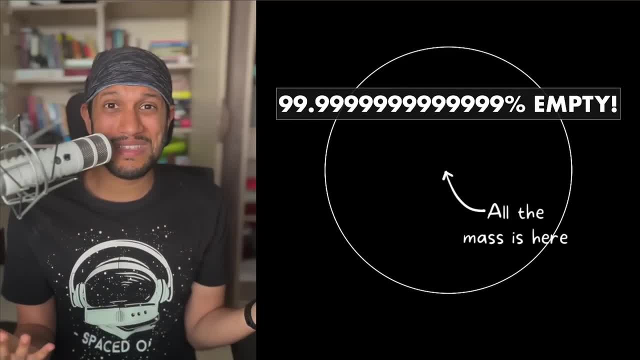 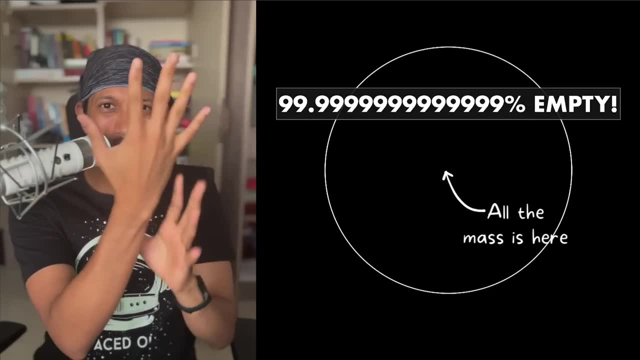 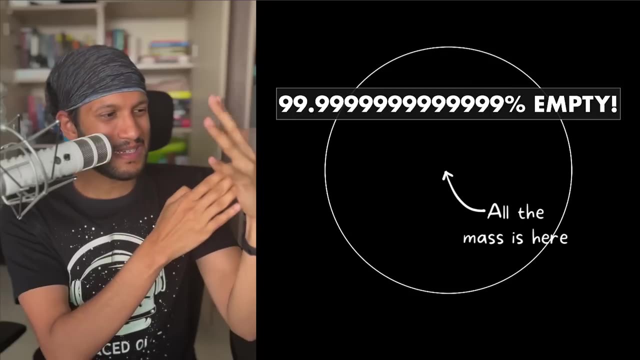 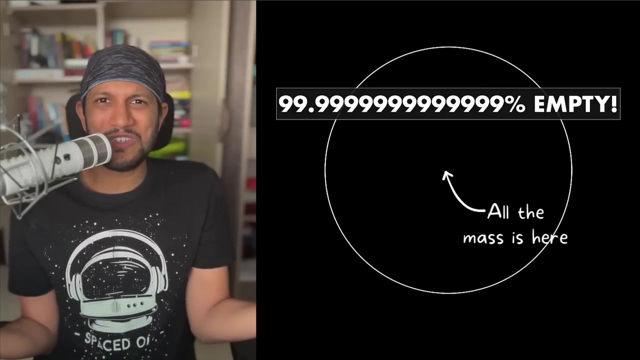 everything that you look around you is just empty space. this also means our brains are empty, and now that makes me wonder: why doesn't this empty hand go through? this empty hand? isn't that a valid question? now, why can't we walk through walls? what gives solid matter its structure? 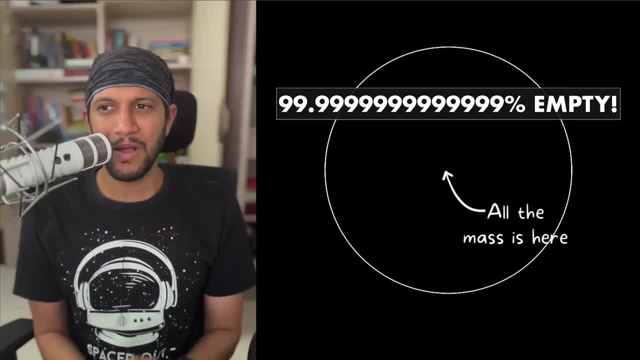 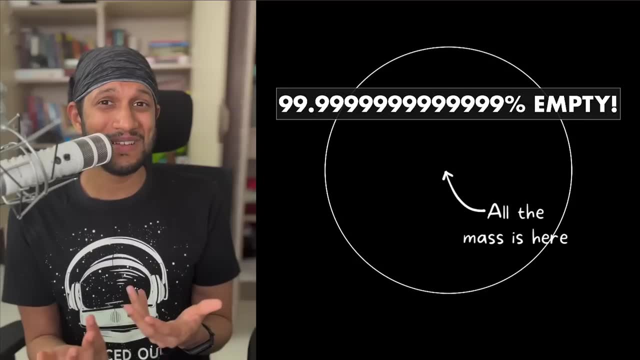 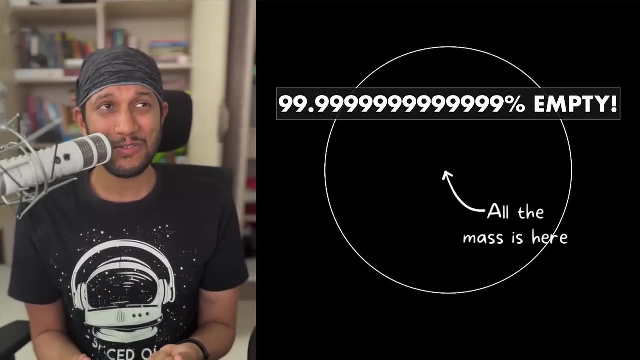 so what's the answer to this? well, patience, I promised you, by the end of the video I'll give you a brand new perspective, and I've done that. hopefully, and hopefully, the question that I've asked also makes sense, sometimes in science, actually, most of the times in science.